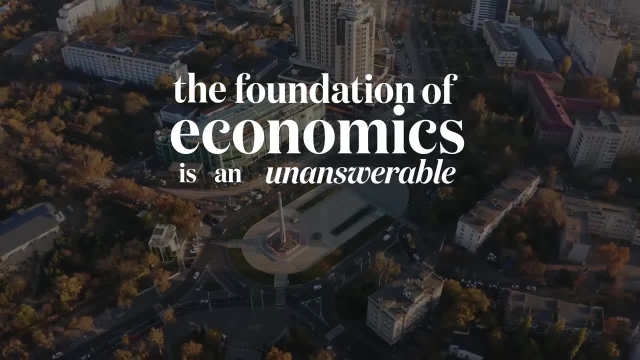 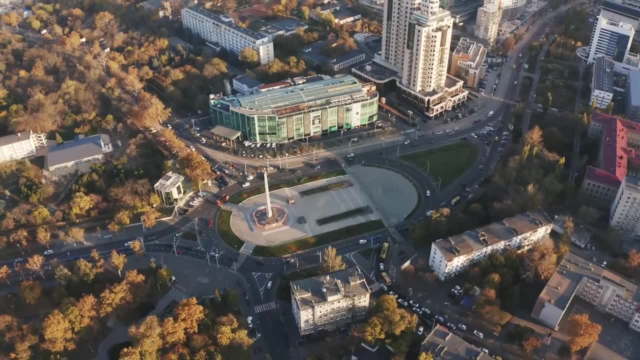 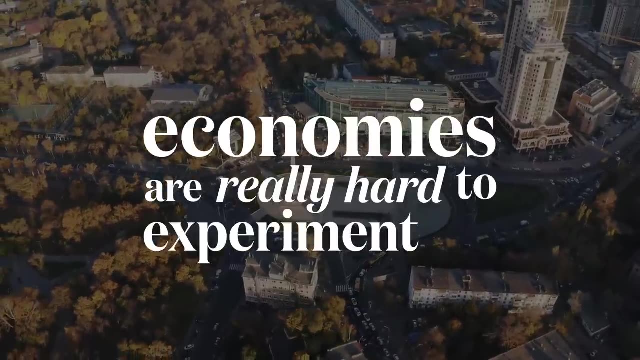 1. The foundation of economics is an unanswerable question, So there is a certain element of philosophy and morality in this academic pursuit, no matter how much economists attempt to sterilize it with mathematics and statistics. 2. Economies are really hard to experiment on If there is some radical new theory about. 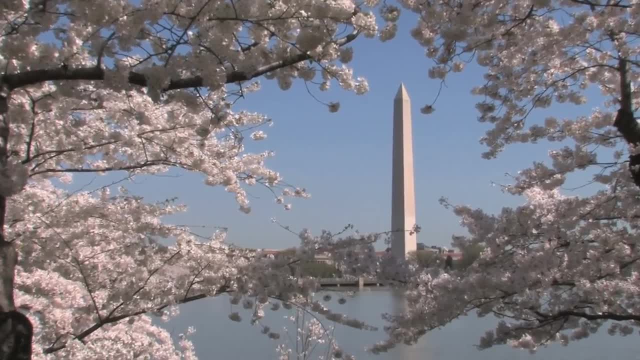 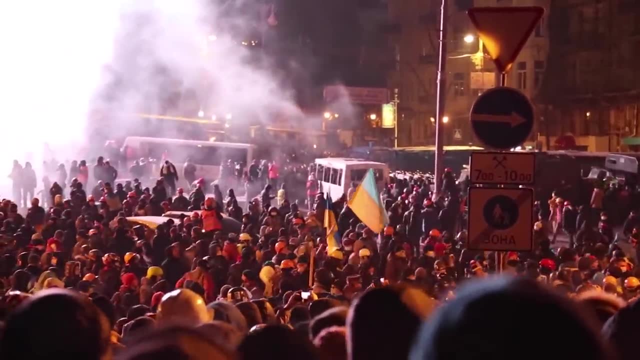 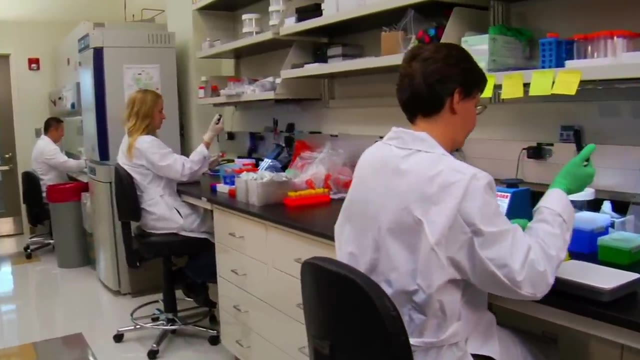 effective taxation. The only real way to see if it will work is to get that tax law passed in a country and study the results. If the experiment doesn't work, then well, you just destroyed a nation. This difficulty in testing also means that a lot of fringe ideas are hard to disprove. 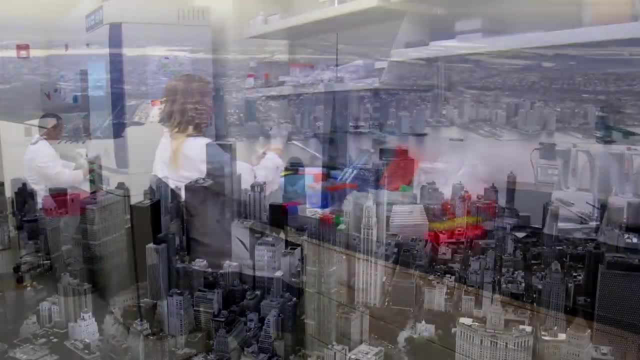 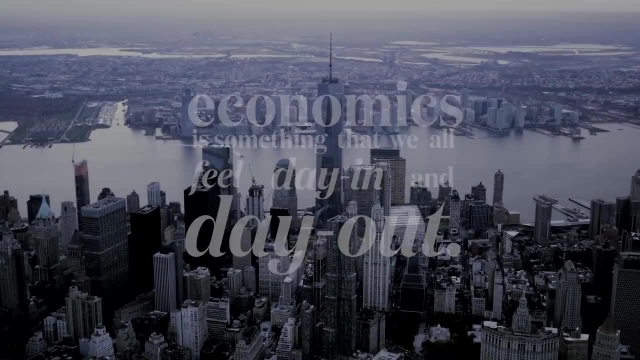 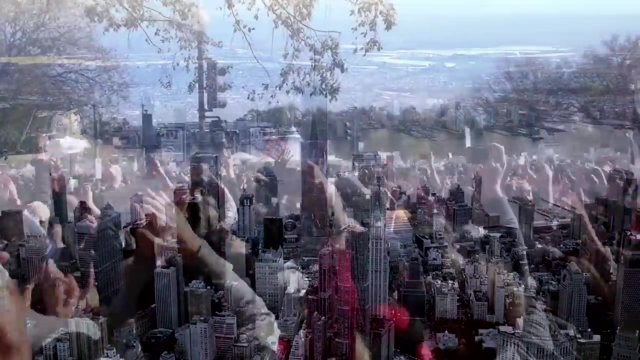 in the same way that they would be in a chemistry lab. And 3.. Economics is something that we all feel day in and day out. The economy impacts our financial situations, our governments, retirements and finances, But you don't have to be such an expert to understand how that can affect your business. 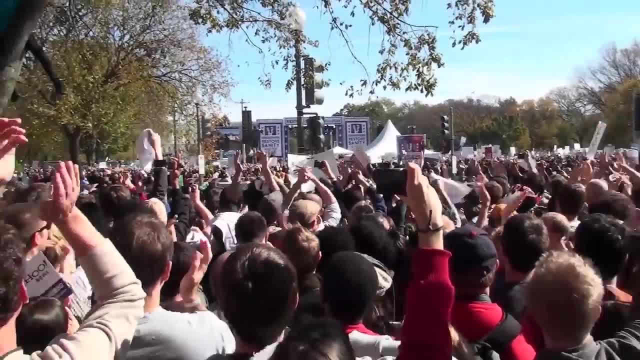 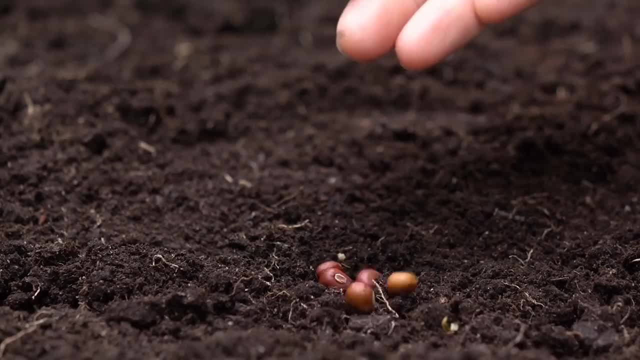 As with everything people are invested in, they form opinions about it, And those opinions are held by everyone, from nobel laureate career economists to that crazy guy advocating for a seed based economy. But if this contention wasn't enough, there is one other issue that makes these schools 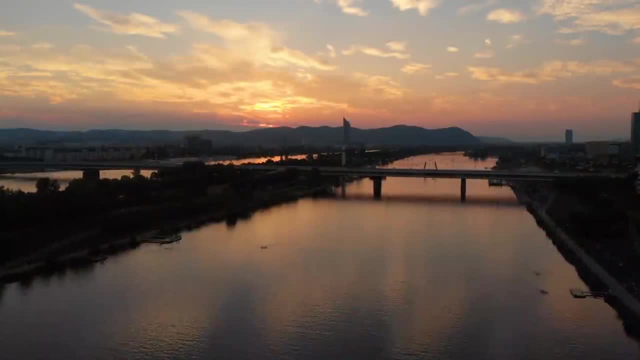 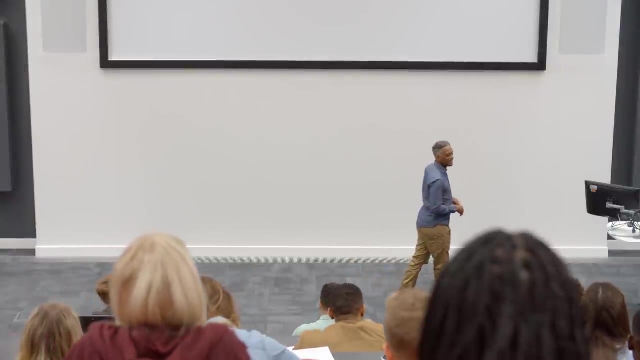 of thought difficult to deal with, and that is there are no strong borders between them. There are plenty of economists that agree with this. There is now a lot of economists in the world who are more interested in the economy than agree with some principles of one school of thought and disagree wildly with some other. 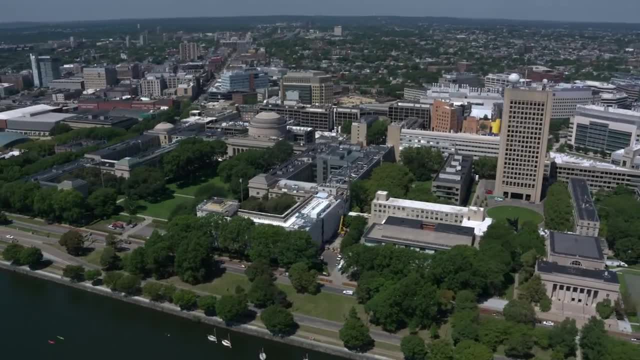 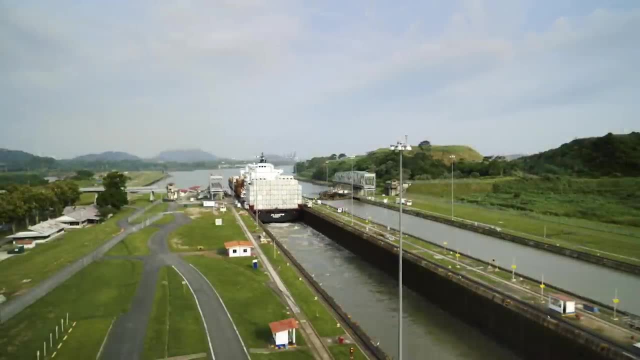 areas, which is actually a great thing. No researcher, in any field, should feel aligned to a certain way of thinking. But for now, to try and make sense of this wild world, we are going to look at three major schools: Classical, Austrian and Keynesian. 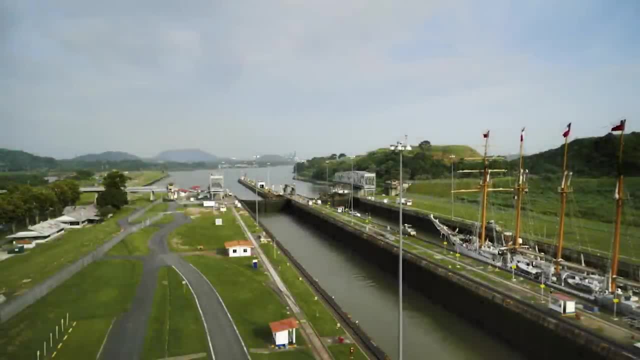 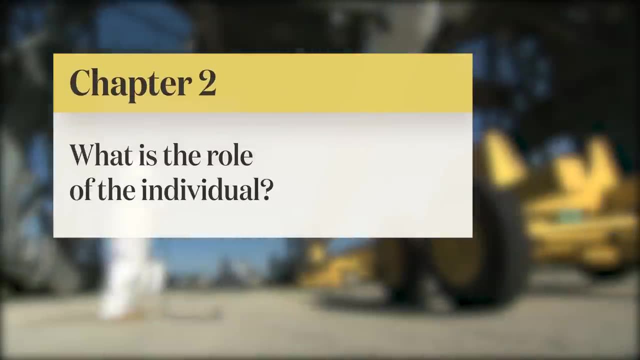 To show the differences between these schools, we are going to look at the way they suggest solving the central economic problem in key areas. What they suggest the role of government is: What do they think the role of an individual is? What do they propose doing during an economic crisis? 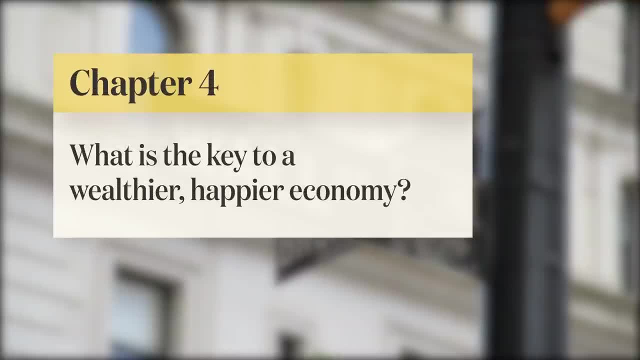 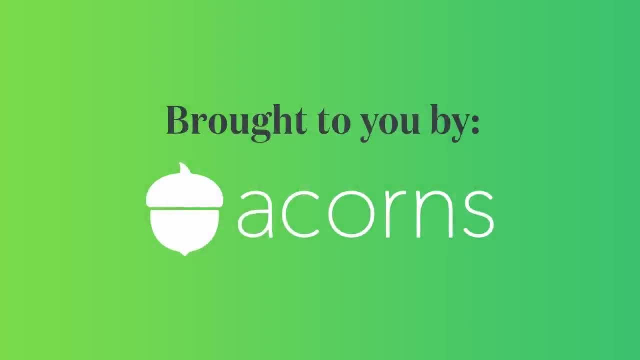 And, finally, what it is they argue is the key to delivering a wealthier, happier economy. The video you're watching right now would not have been possible if it wasn't for our amazing sponsor, Acorns, an investment app that automatically rounds up your credit and 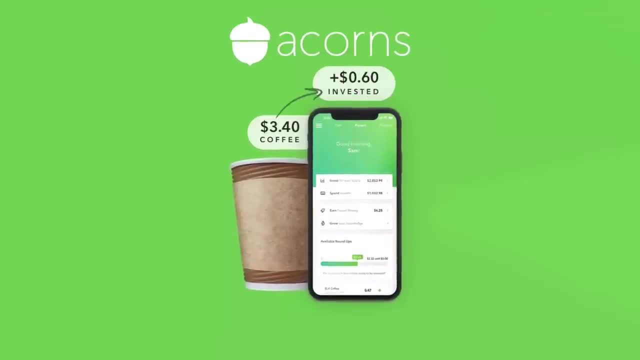 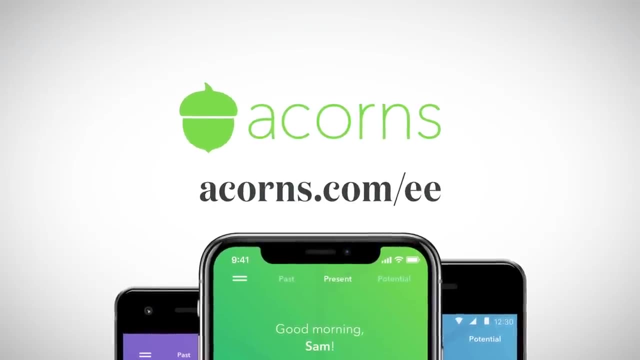 debit card purchases to the nearest whole dollar and then auto invests the spare change for you into a diversified portfolio. Sign up now by going to acornscom, Acornscomau, Or click the link in the video description below, and acorns will deposit $5 into your. 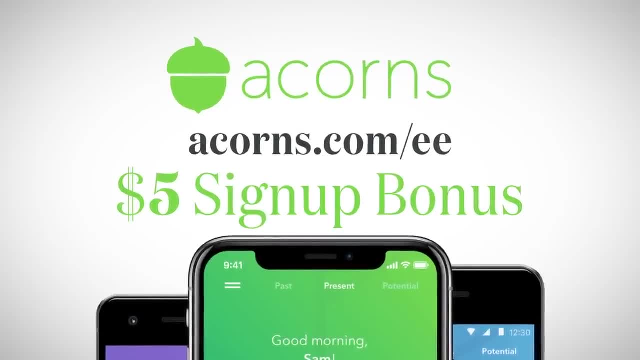 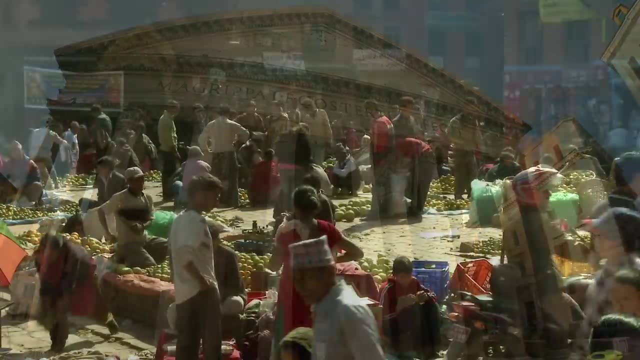 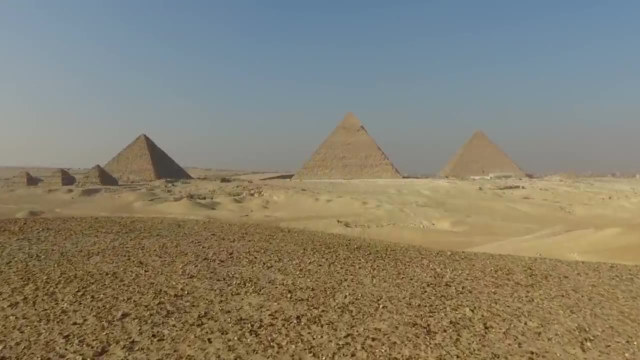 account to help you get started. That's acornscomau. Now, economies have always been a thing, and before people even knew what they were doing, they were attempting to satisfy their desires with the limited resources they had available to them. This went on for an extremely long time and great empires rose and lived and died all. 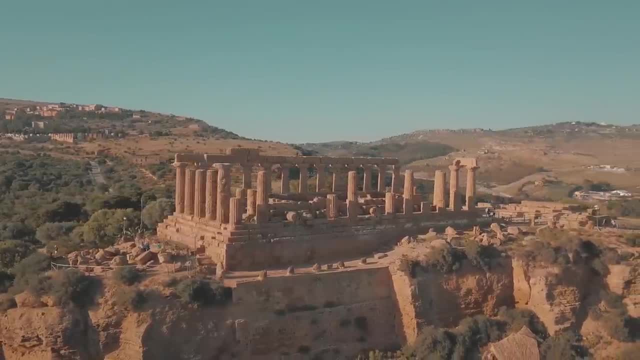 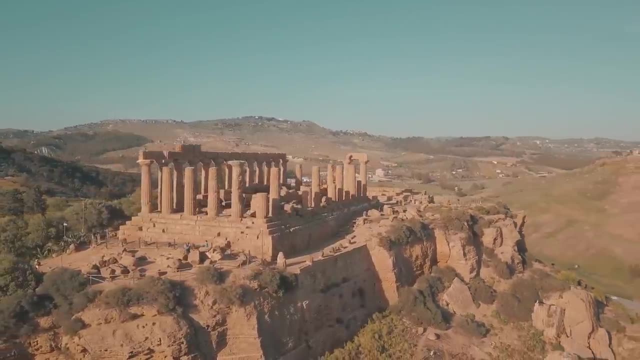 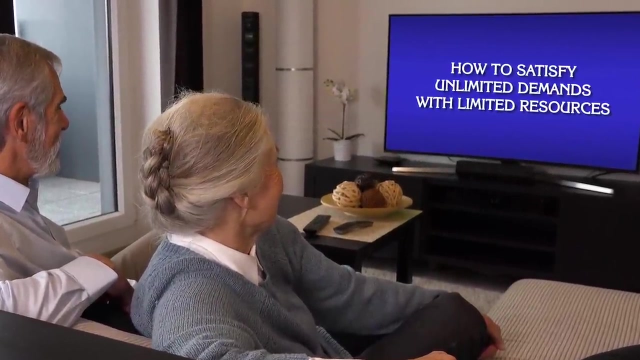 while harboring economies that they didn't think to themselves. The only way to find out was through research. Everybody, from Aristotle to Jesus, presented an answer to the question, but nobody had yet thought to ask what the question was. Ah, yeah, can I have how to satisfy unlimited demands with limited resources for 1000 alex? 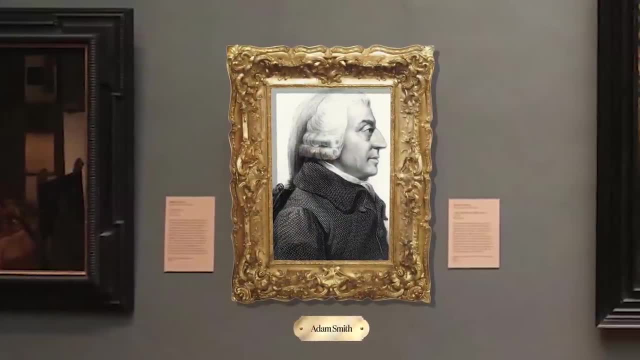 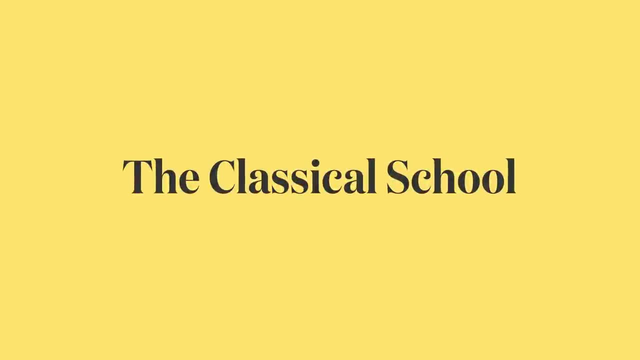 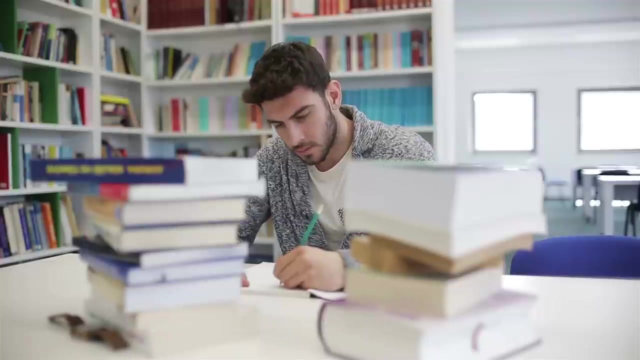 This all turned around, though, in the 18th century, with a man called Adam Smith, who gave birth to economics and formed the foundation of what is now known as the classical school. The classical school- of economics- name would suggest- was the first incarnation of economics as a separate academic pursuit. 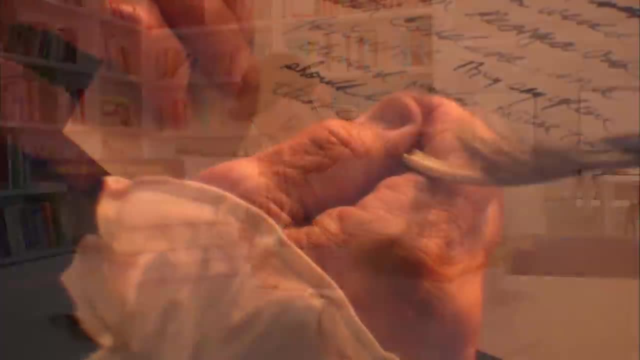 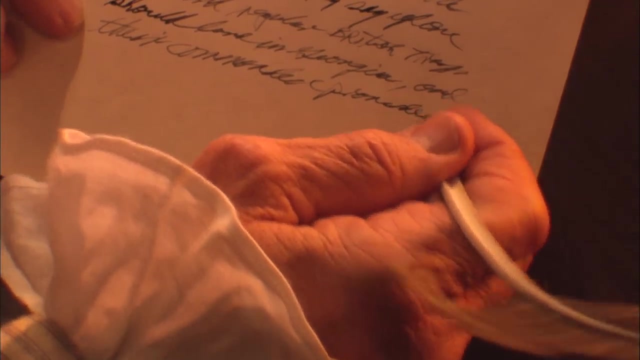 Distinct from finance, government and philosophy. the early practitioners of economics, namely Adam Smith, started writing and studying about how the world was operating to increase the wealth of nations. They found that the world at that time was ruled by a theory that went on. 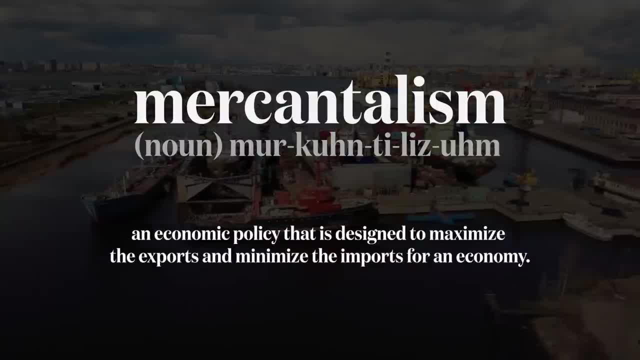 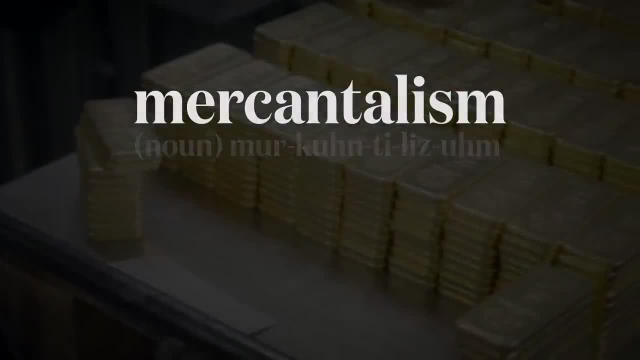 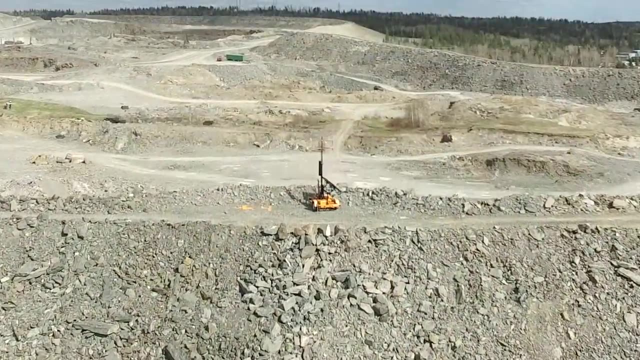 to be known as mercantilism, which could realistically be its own economic school of thought, had it not been so fundamentally flawed. This system relied on nations just desperately trying to hoard as much gold as they could by either exporting more than they imported, mining more of it within their borders or 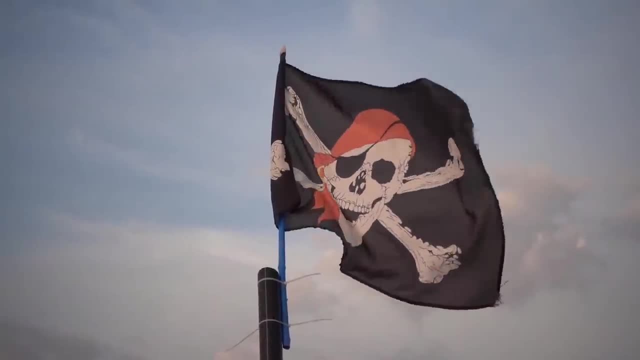 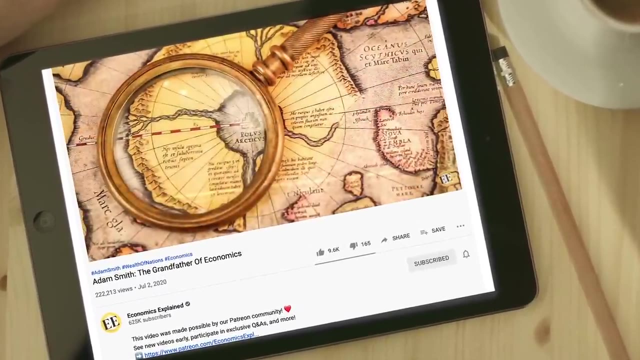 their colonies or by plundering it through hostile conflict. Now we have explored mercantilism and Adam Smith before on this channel, so if you want more insight on that, go and watch those videos. But the big takeaway here is that mercantilism was realistically. 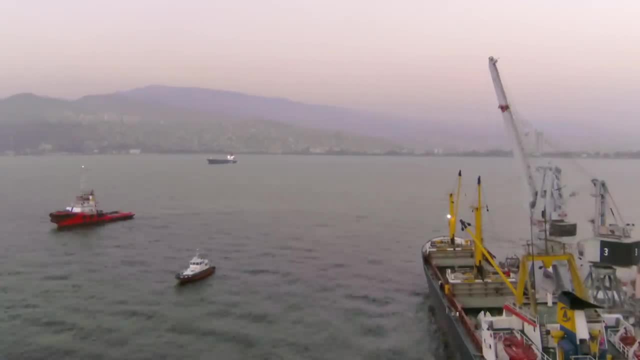 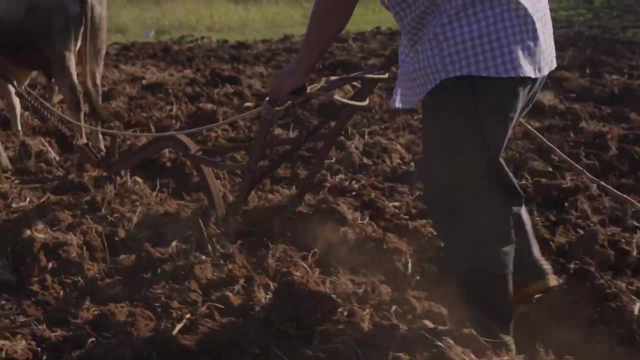 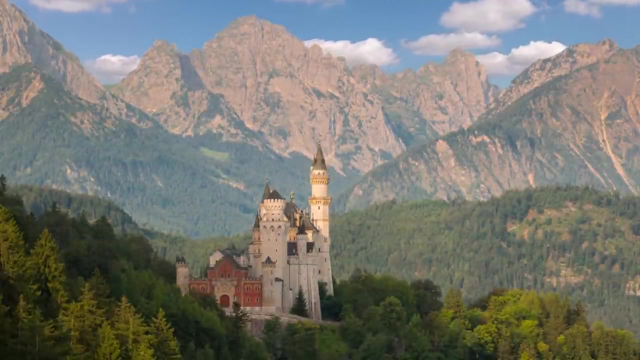 just fine for mercantilism. Most nations throughout history, These nations were extremely basic and their economic success primarily revolved around the strength of their harvest at any given year and later turned into how many colonies they could claim More or less. it was a zero sum game If someone or some country was getting richer. it was because someone else or some other nation was getting poorer, and mercantilism perfectly mirrored this reality. Having a perfectly run fiscal and monetary policy would not have meant very much to the overall prosperity of these types of very basic nations. It would have been like putting nitrous oxide on a horse drawn carriage. 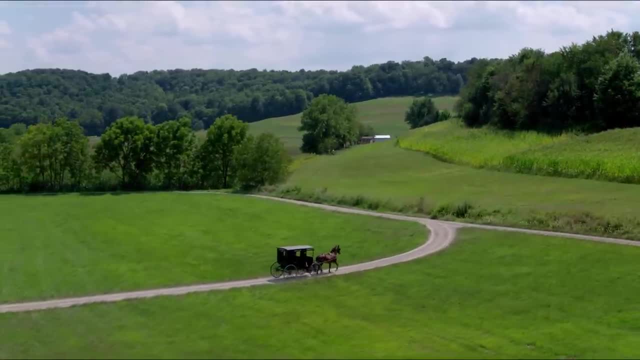 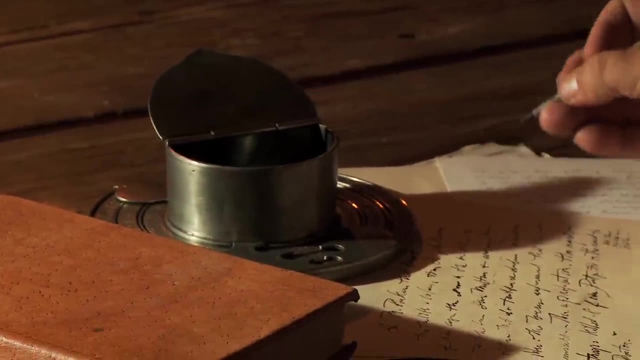 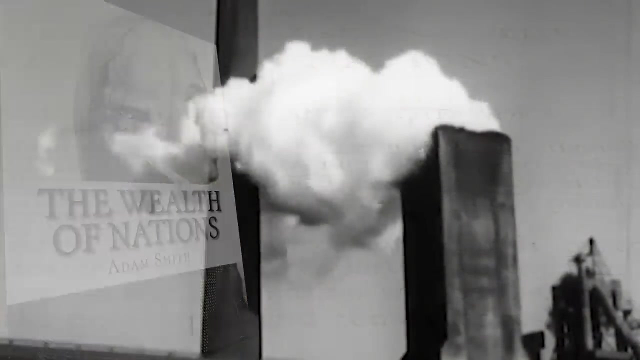 It wasn't going to do anything, and it would probably just make everyone very confused with its needless complexity. This was all starting to change, though, when Adam Smith was putting pen to paper to write the wealth of nations. The first steam powered factories had sprung into existence, and, for the first time ever, 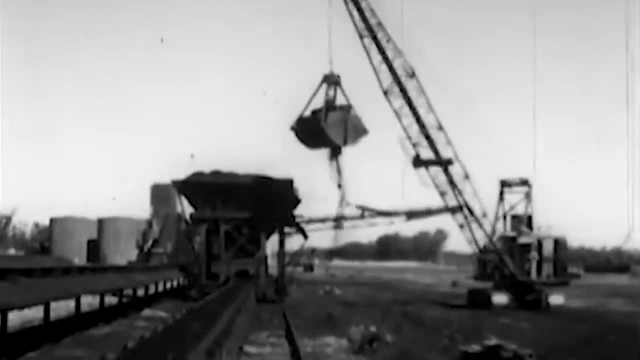 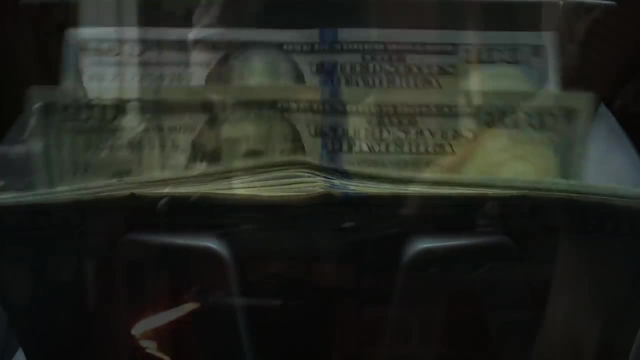 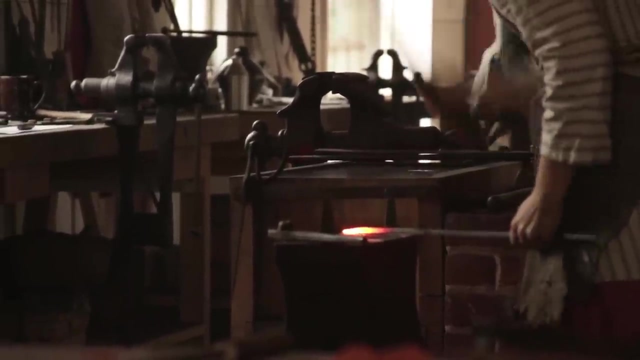 wealth was not being grown, It was being created en masse, which was a chance for all people to become wealthier. No society can surely be flourishing and happy of which the greater part of the members are poor and miserable. It is but equity, besides, that they who feed, clothe and lodge the whole body of the 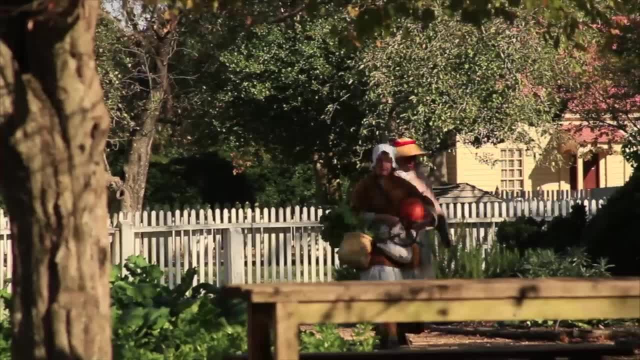 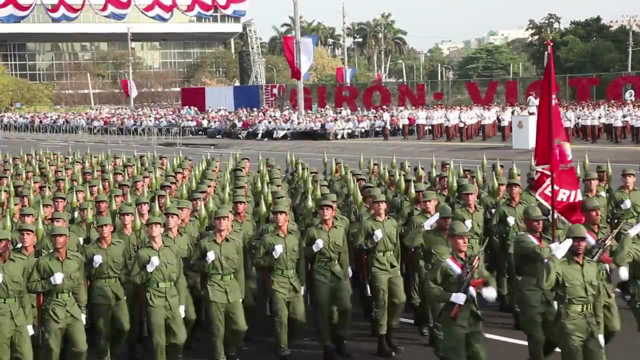 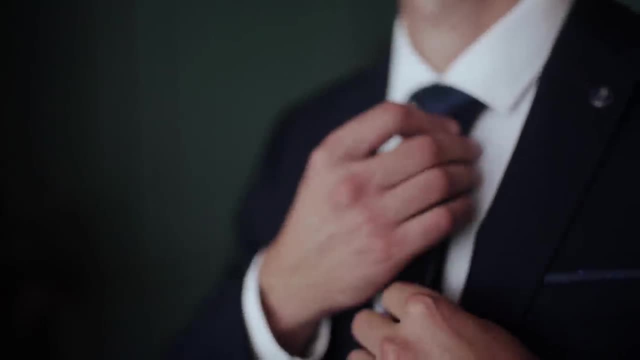 people should have such a share of the produce of their own labour as to be themselves tolerably well fed, clothed and lodged. Now this sounds like some commie nonsense, but what Smith was trying to say here is that there is an optimal distribution of wealth creation for all members of society. 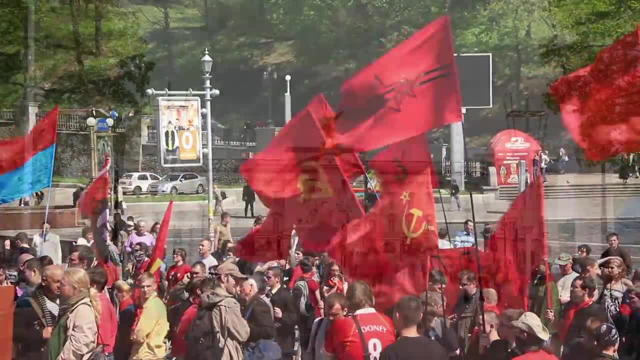 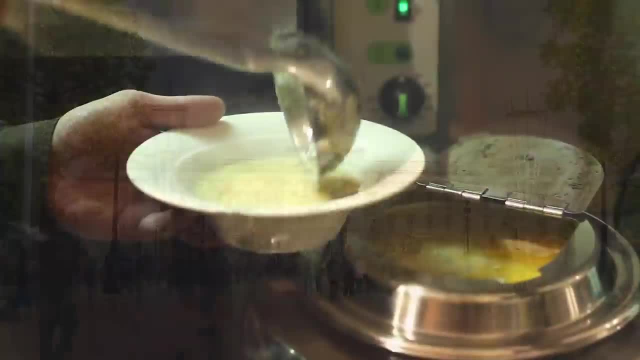 It definitely should not be completely equal, but it shouldn't be a swelling peasant class holding up a tiny nobility either. The reason for this was not some virtuous quest to feed the poor, but rather it was to develop markets and divide labour. 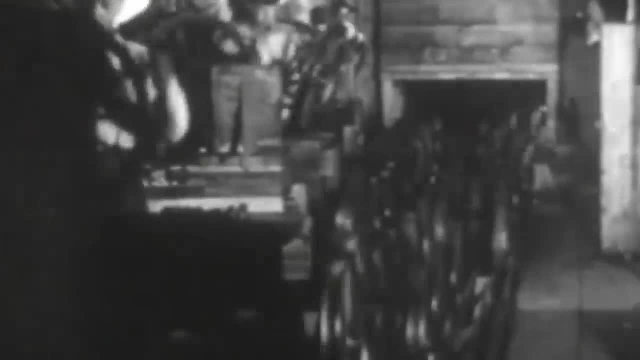 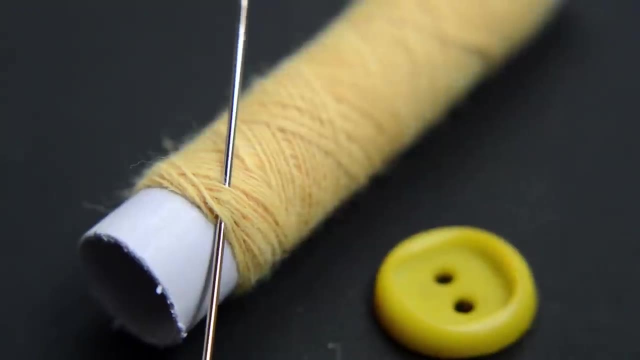 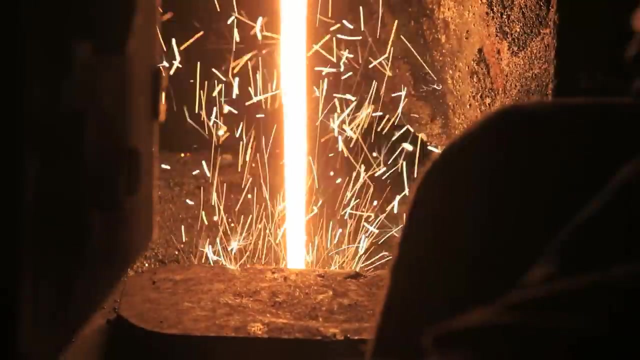 To show the importance of this, Smith used the example of a pin, A small, sharp pokey metal stick, Which sounds like an extremely simple product. But if a single worker was to wake up in the morning and dedicate themselves entirely to making one single pin, they probably wouldn't be able to do it. 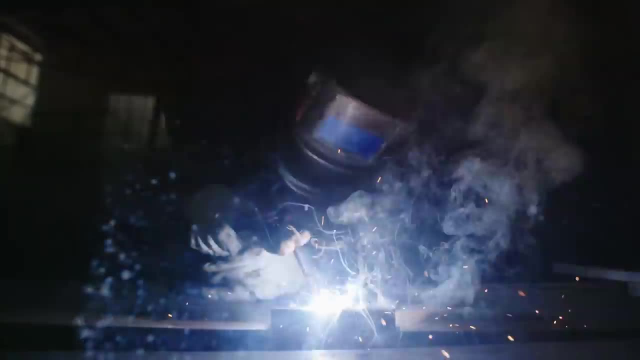 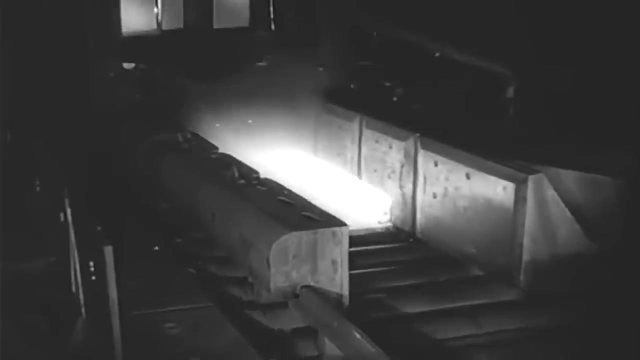 because they would need to mine the materials, refine the steel, forge it and then sharpen it just to make one pin. Of course, if all of these tasks were done by separate workers, then they could just focus on their individual role and produce a pin, But producing pins would become a lot easier. 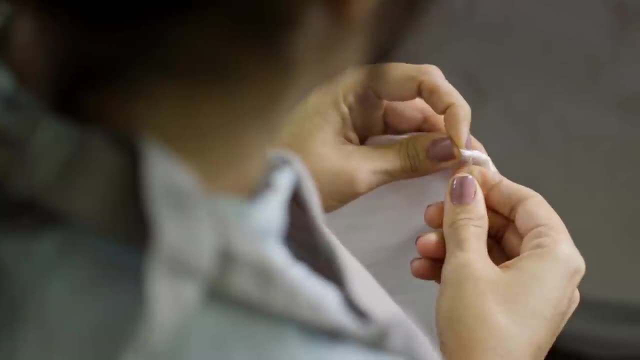 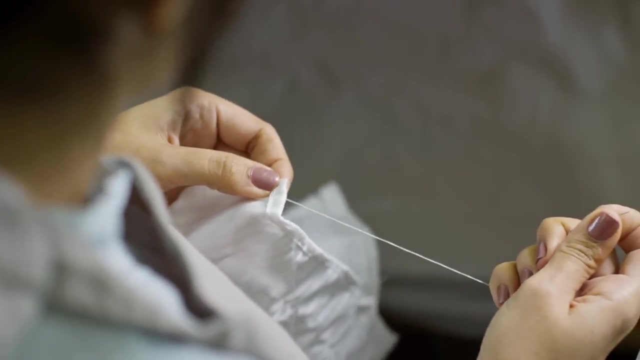 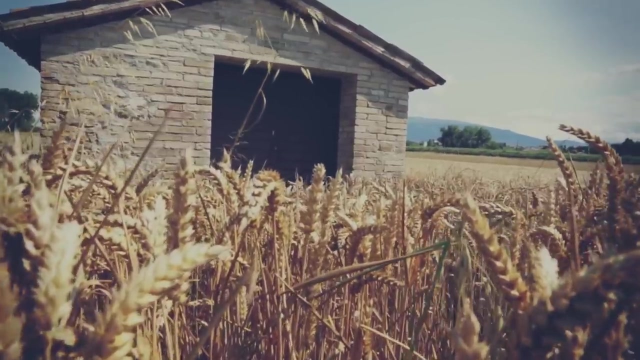 So much so that there would be an abundance of pins that they could then share around between all of them, and everyone would have more for having contributed to this process. Now, this example of one person making a pin sounds pretty silly to us, But for a long time, this was effectively how economies operated. 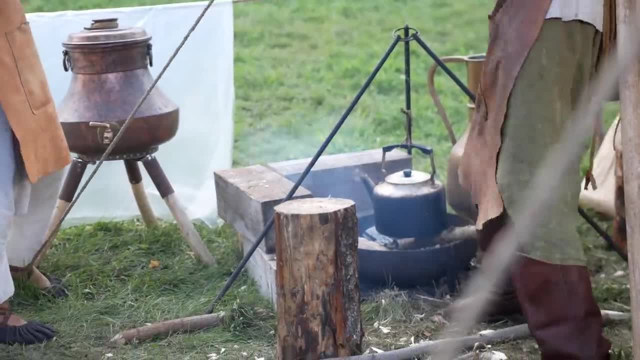 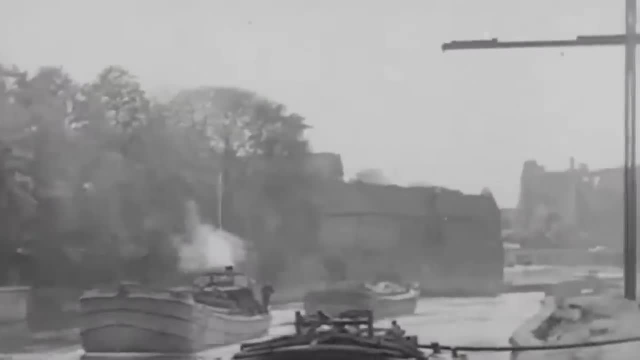 Feudal villages would produce pretty much everything they needed, and even individual households would be more or less self sufficient. The reason why people did this is because they were not the only ones who were able to produce this. They didn't have any real alternative. 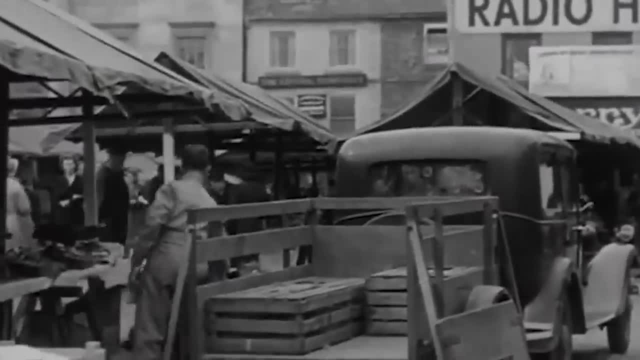 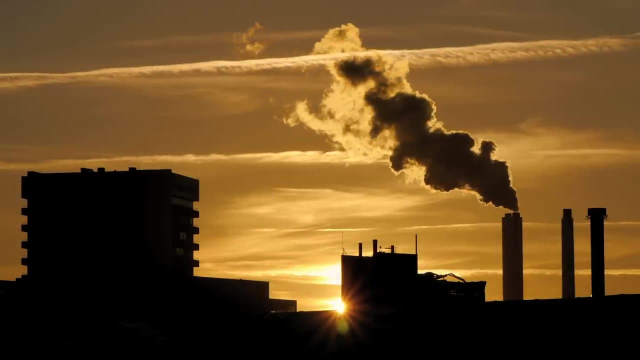 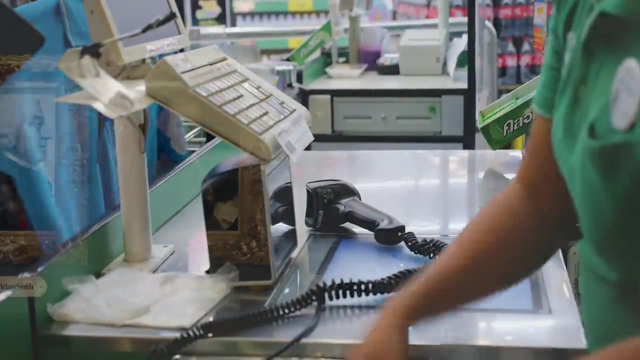 Village markets were basic at best and most peasant workers didn't even receive an income as you or I might know it today. But by moving into factories and earning a cash wage, individuals now had the ability to make purchases, which gave the entire economy the ability to specialize. 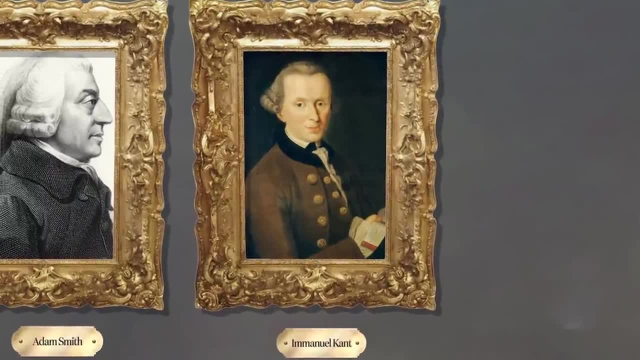 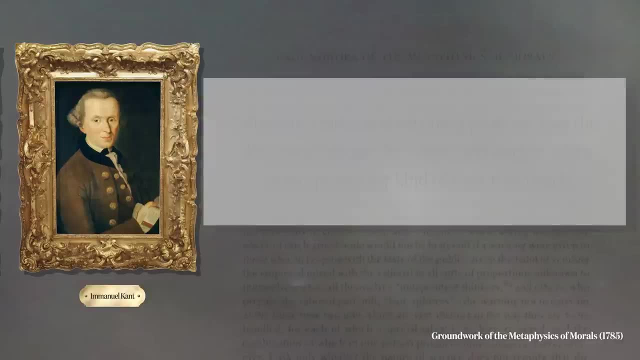 Immanuel Kant, a legendary philosopher of all people, may have said it best in his 1785 book The Groundwork of Metaphysics and Morals, where he quoted that all crafts, trades and arts have profited from the division of labor. 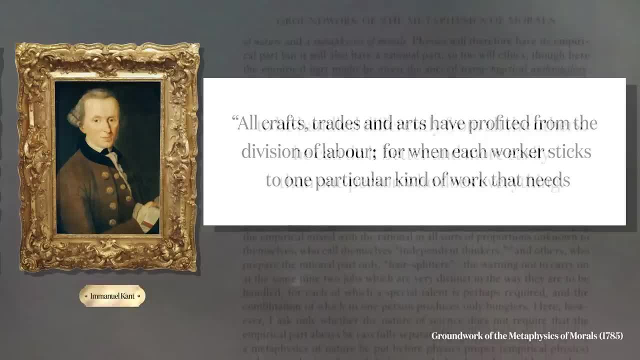 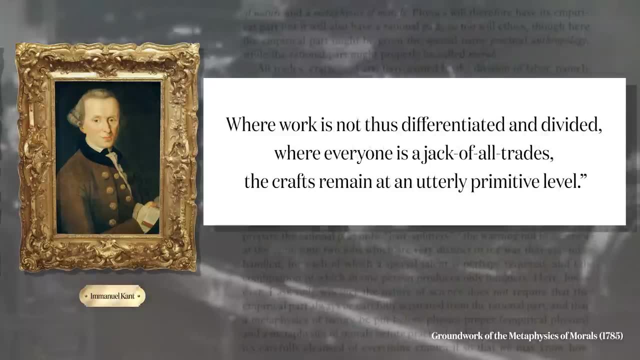 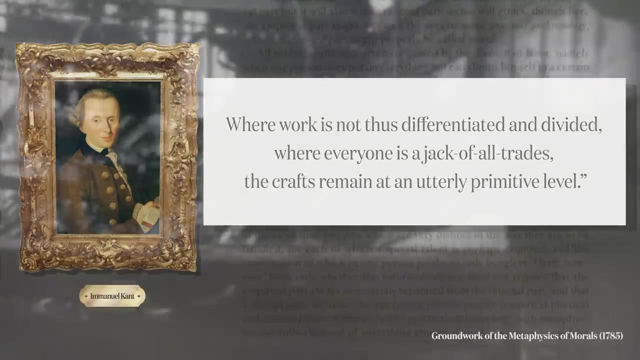 For when each worker sticks to one particular kind of work that needs to be handled differently from all others, he can do it better and more easily than one person who does everything. Where work is not thus differentiated and divided, where everyone is a jack of all trades, the crafts remain at an utterly primitive level. 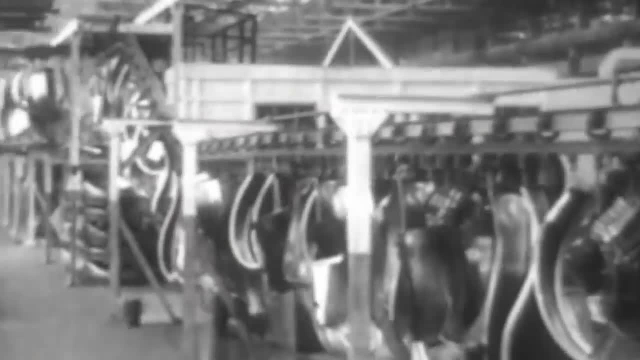 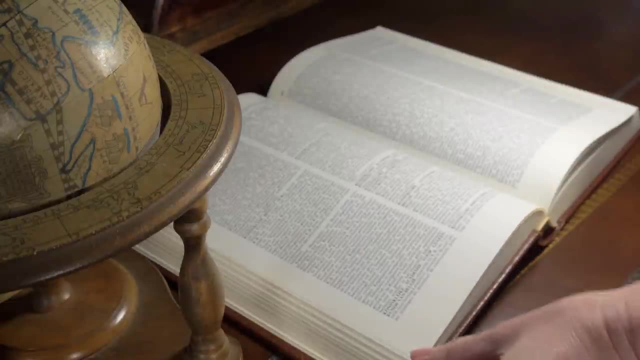 So, with this new understanding of how to build a better world. these were the prescriptions of these early philistines. They were the ones who were able to make the most of their work. Philosophers and Financiers Turned Economists. Markets should be free, because the more that people are allowed to trade freely with one. 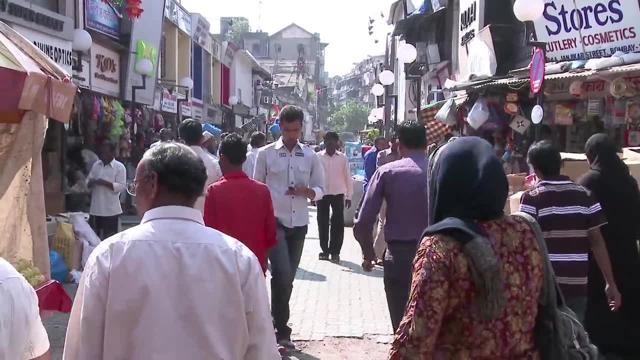 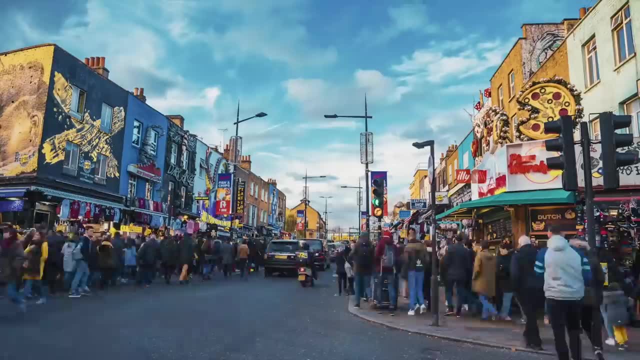 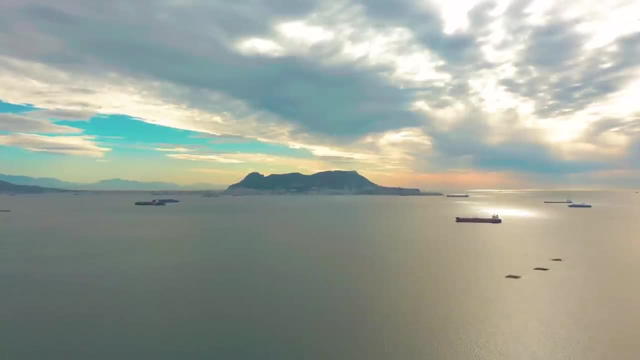 another, the more they can specialize and count on others to specialize to deliver all of the goods they may need. Nations should also do the same thing. Stop trying to hoard all the gold and instead take note of who does what well. Once this is known, trade amongst other nations to increase overall wealth. 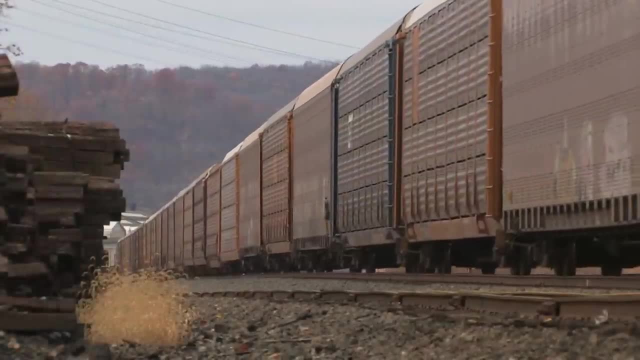 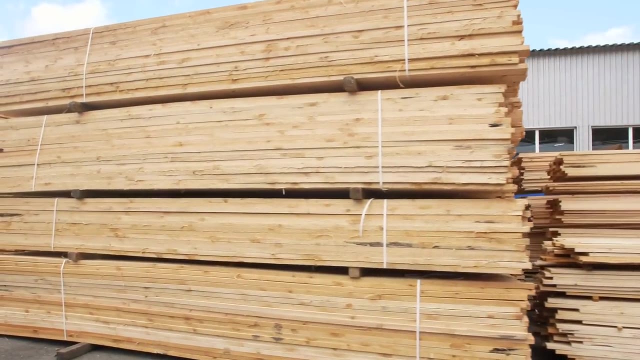 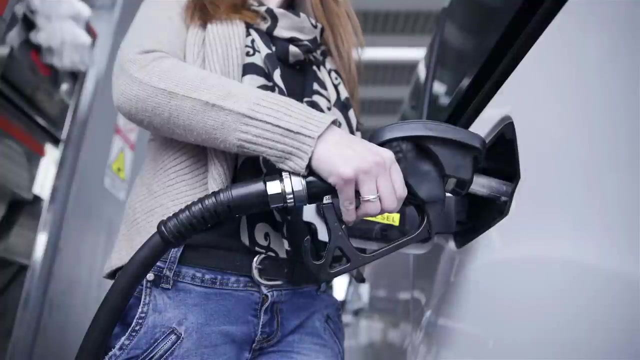 Production is the most important part of an economy, and great efforts should be made to making this more efficient so that more wealth can be created from turning raw materials into complex products. Government intervention into free markets should be limited exclusively to making sure that contracts are upheld and fraud is not allowed to take place, and of individuals. 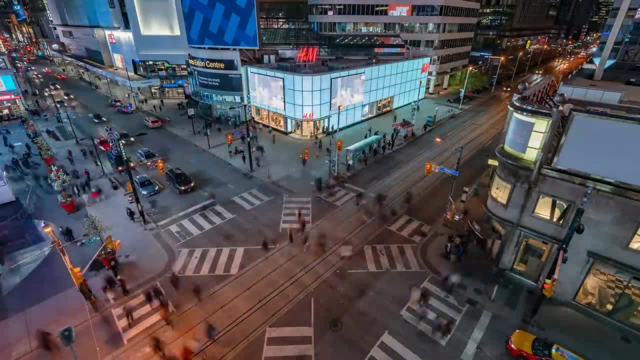 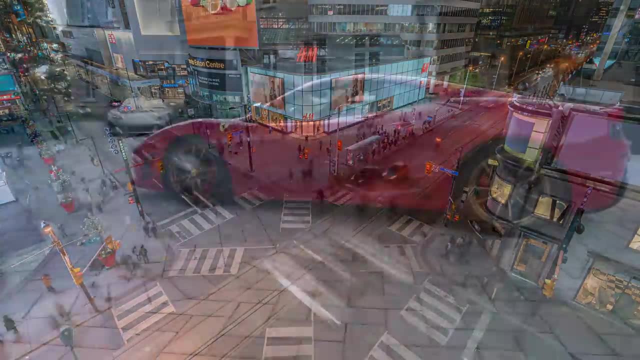 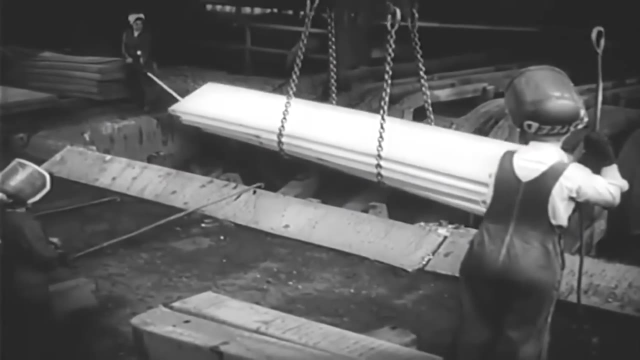 Classical economics assumes that everybody buying and selling and working is a perfectly rational individual and will always make the most logical decision possible to forward their own selfish interests. More or less classical economics argues that we could all work together to make the world a better place by being extremely selfish. 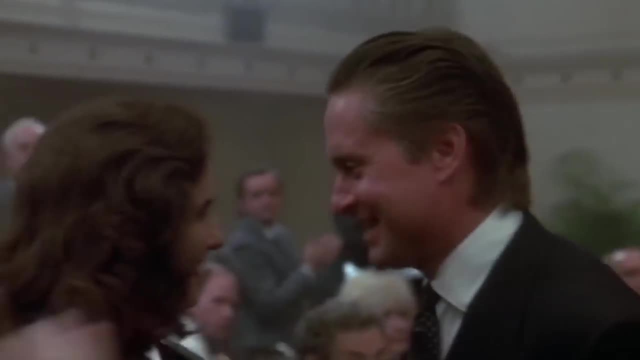 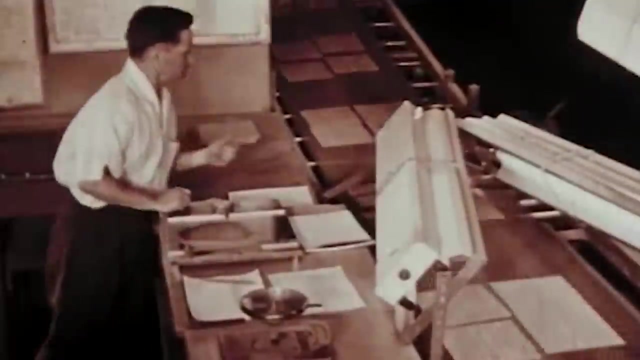 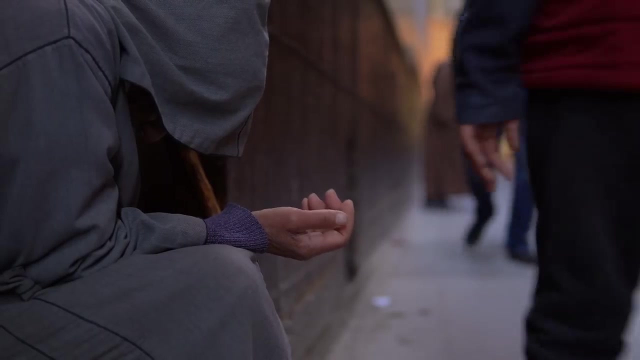 I guess Gordon Gekko was probably a classical economist. Now, these theories worked very well and when applied to the age of industries, they were the guiding force behind the development of jobs, companies and markets as we know them today. But these ideas weren't perfect and now that the 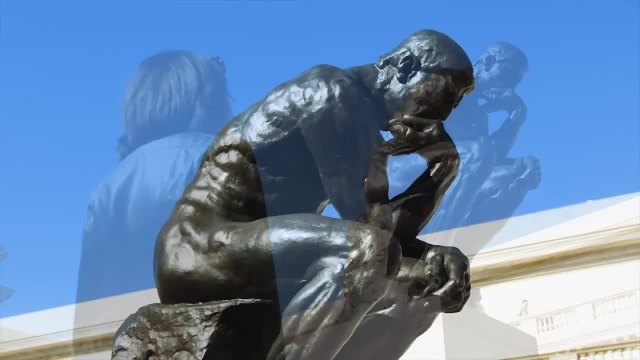 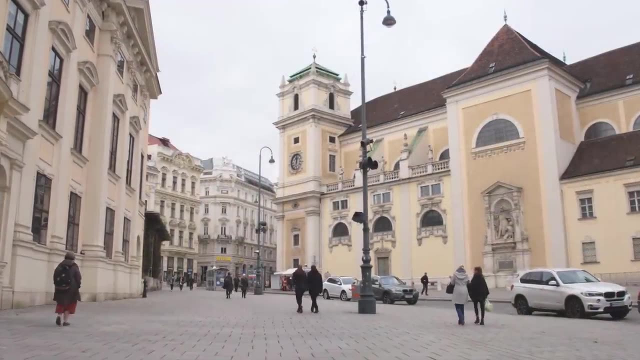 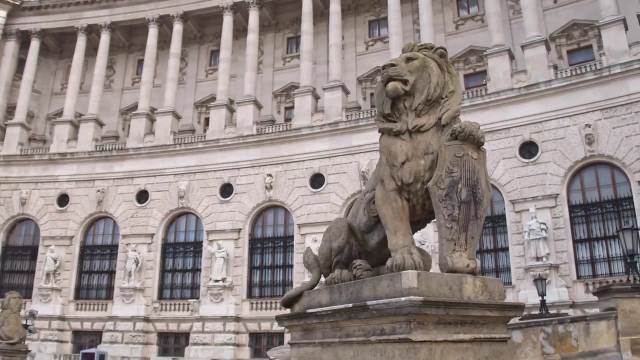 foundation was set, the great thinkers from around the world got stuck in on how to improve it. The first to really shake up this new way of thinking were a collection of economists from Vienna who went on to form the Austrian school. The Austrian school shares a lot of similarities with classical economics and most of the 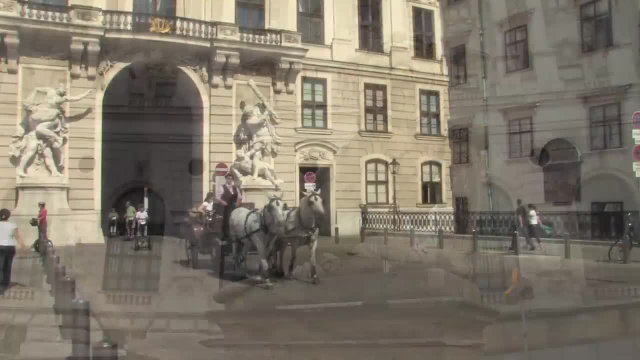 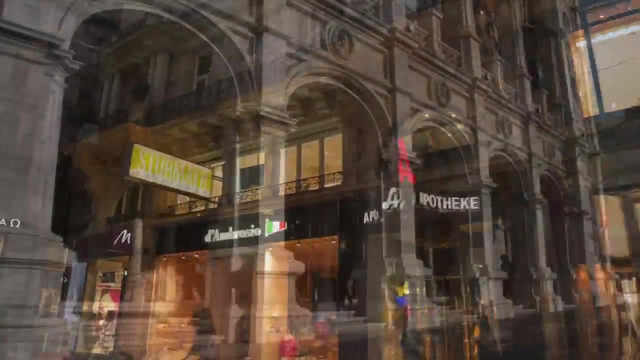 economists that have now gone on to define this particular school of thought didn't even know that they were forming one, in the same way that Adam Smith probably didn't even know he was creating the discipline of economics. Rather, these early academics were trying to fix up some loose ends of classical economics. 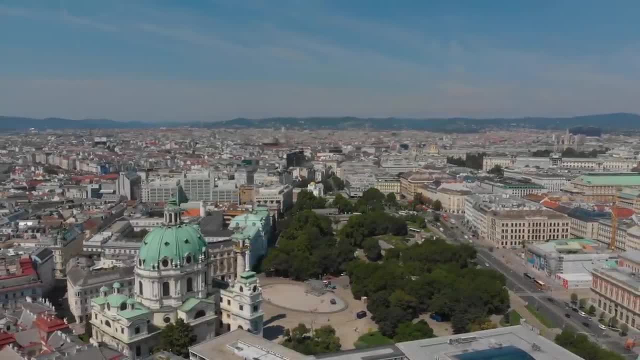 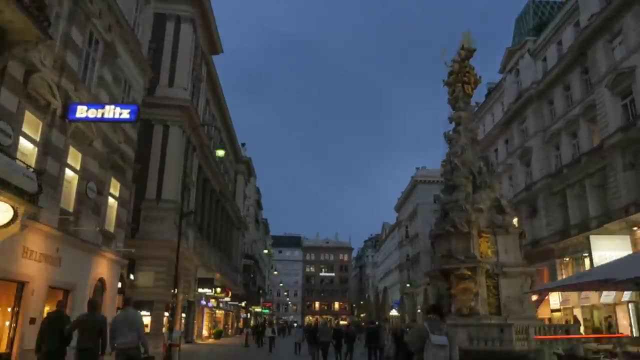 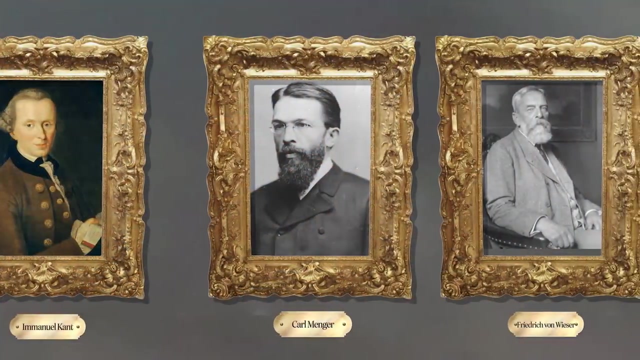 primarily by realising that an economy wasn't some amorphous blob of production, but rather it was a collection of individuals. With this, these scholars started adding in more allowances for how individuals acted and specifically how they valued things. Karl Menger was the father of the Austrian. 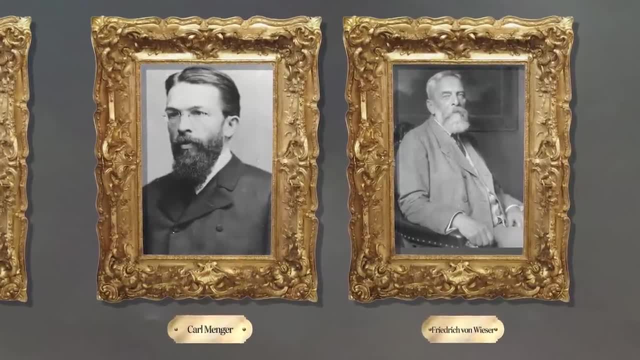 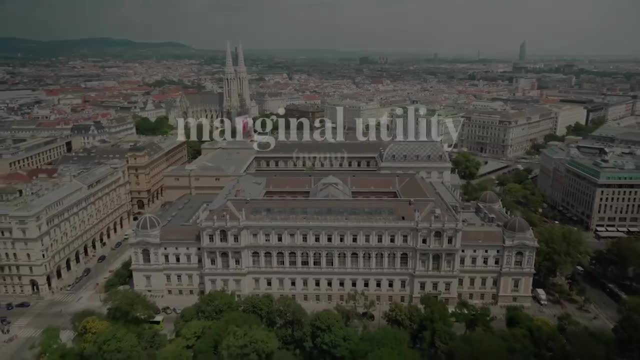 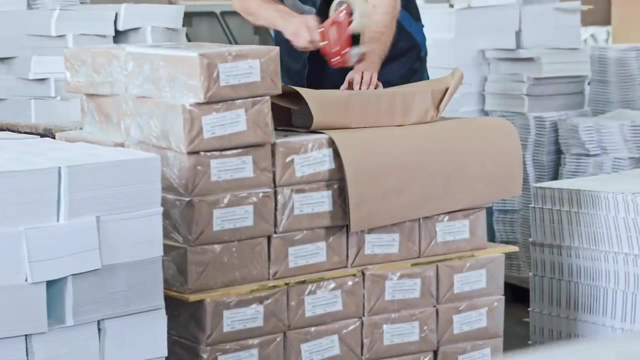 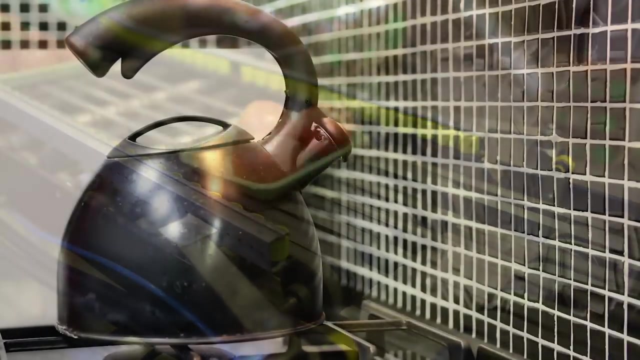 school of economics and is credited with contributing to the theory of marginal utility Alongside his student, Friedrich von Weisser. the theory of marginal utility was an extremely important contribution to economics as a whole. It argued that goods provide a utility, but their utility is decreased for every extra unit of good that there is, For example, the extra utility 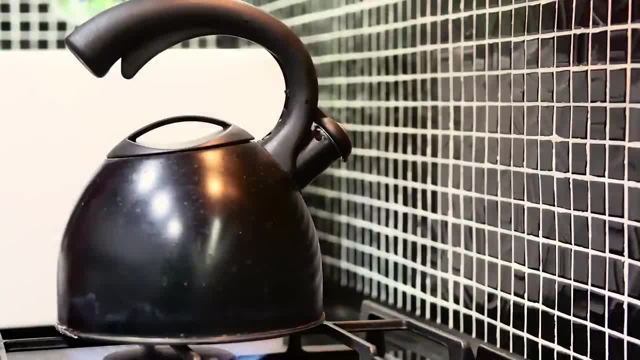 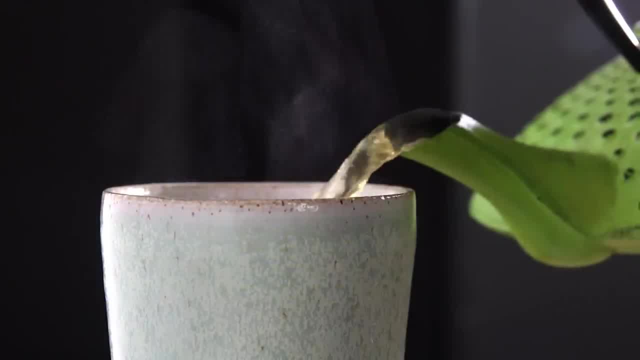 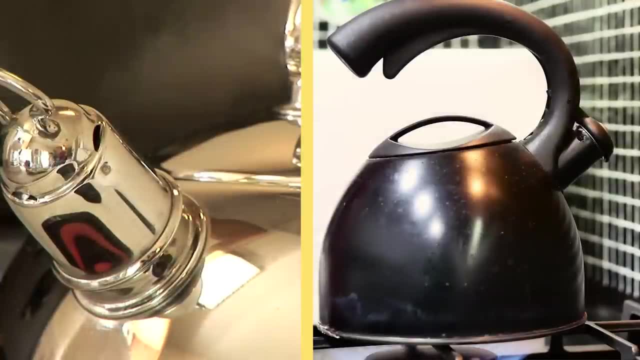 someone gets from having one kettle as opposed to zero kettles is pretty big. Suddenly they can boil water and make tea or coffee where they wouldn't have otherwise been able to in the future. Going from one kettle to two kettles also has some benefits. You can now boil more water at any. 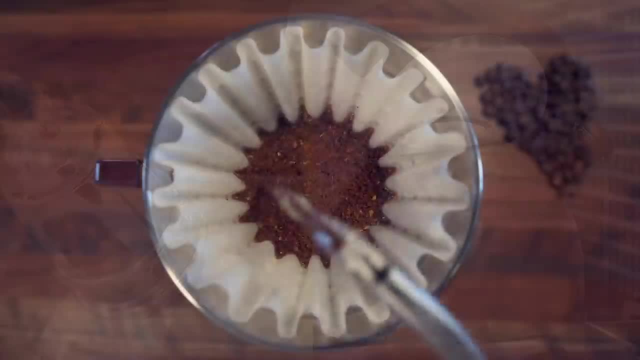 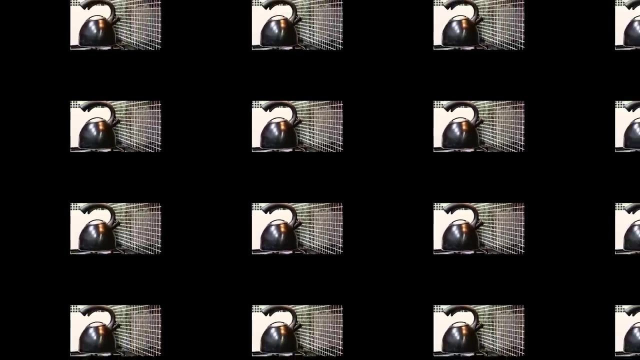 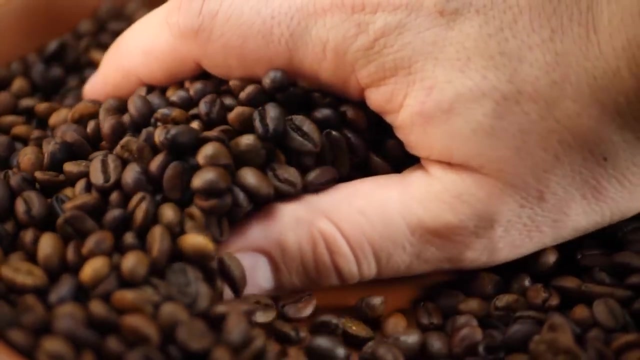 given time and if one breaks down you have a spare there, ready to go for redundancy, ready tea and coffee making duties. But 3 kettles, 4 kettles, 20 kettles- There is only so much tea and coffee a household really needs- and eventually these items start taking up so much space. 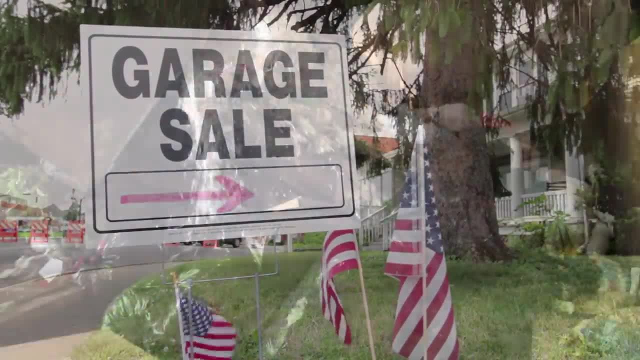 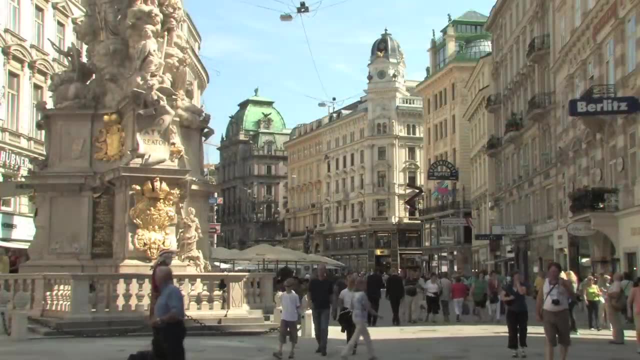 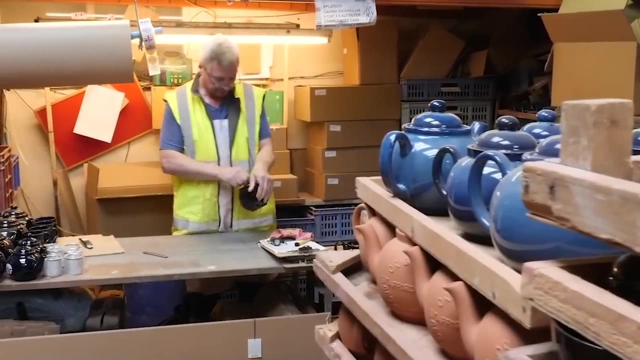 that people want less of them, meaning that at extreme levels an item can have a negative marginal utility value to a consumer. This ran contrary to the classical school of economics, which simply advocated for making as much stuff as possible and then letting the free market decide where that stuff went. 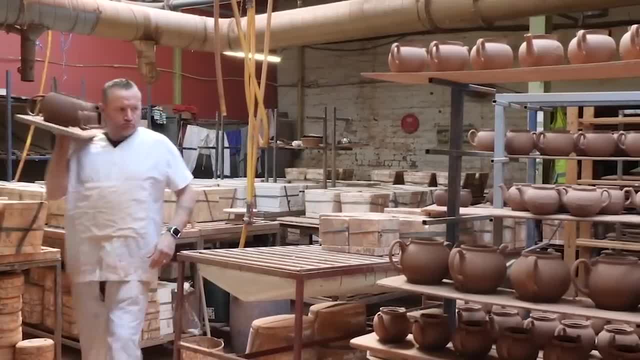 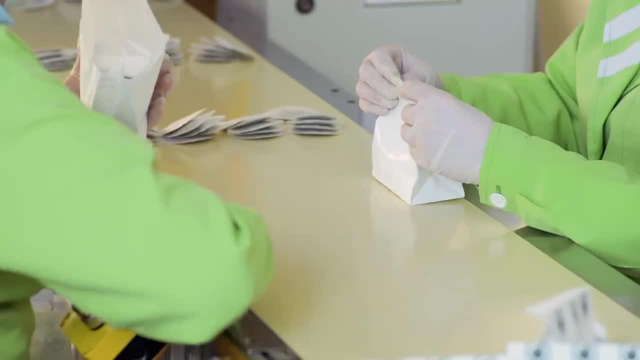 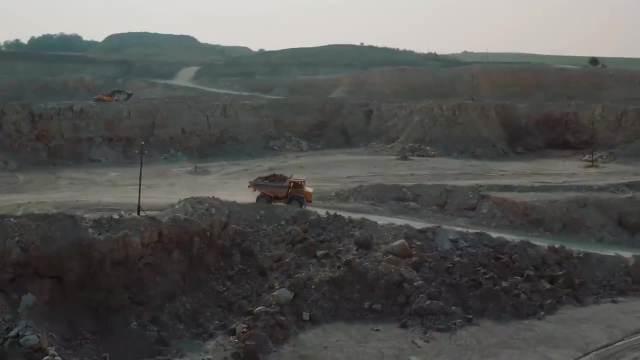 Now again. this might sound obvious to us now, but you have to remember two important things. The first was that this theory made huge contributions towards solving the central economic problem. Sure, they still had unlimited desires and only limited resources in which to fulfil those desires, but they added the asterisk that 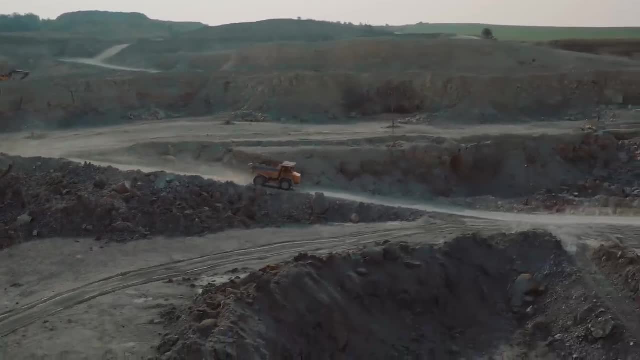 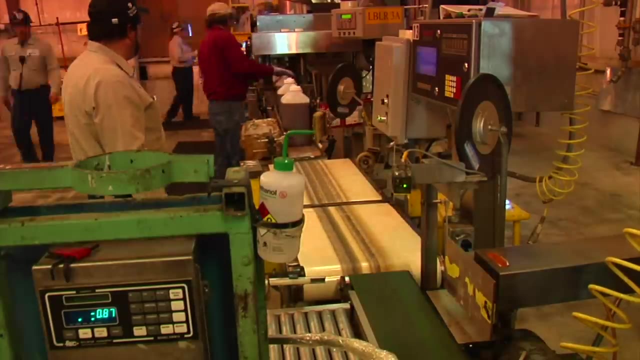 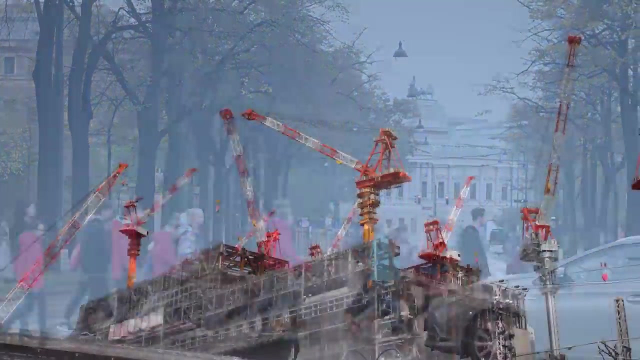 actually, some specific desires can be over satisfied, so an economy must avoid these at all costs, where there is more left over to satisfy other desires that haven't yet been met. The second was that this was the first inkling of an economic theory adapting to a world of genuine 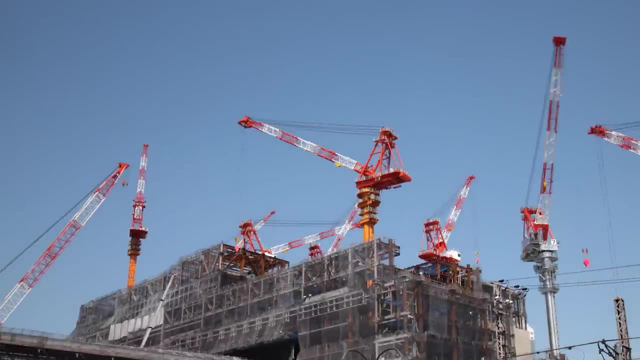 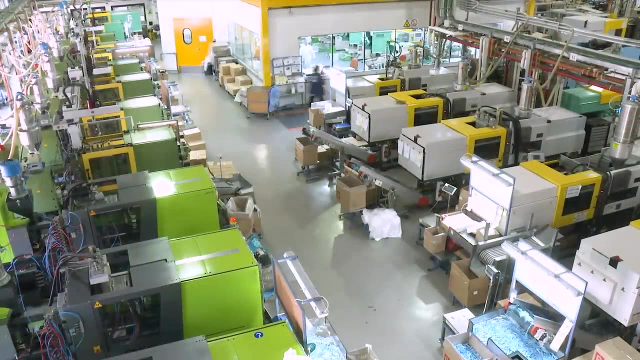 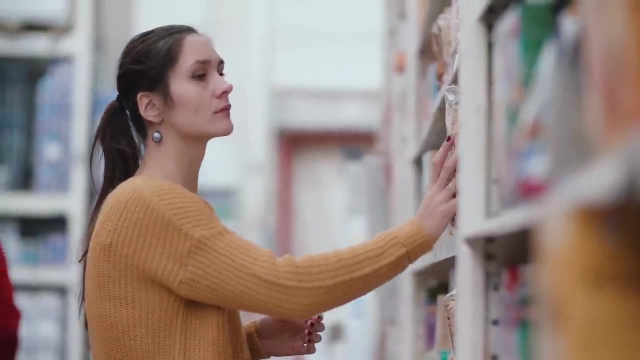 sustained growth. Before the 1800s, the idea that anybody could have too much of something was pretty bizarre. But with factories all across europe working day and night to produce all manner of everything, the decision that everybody was making was starting to shift from: can I afford this to? would I rather have this or that? 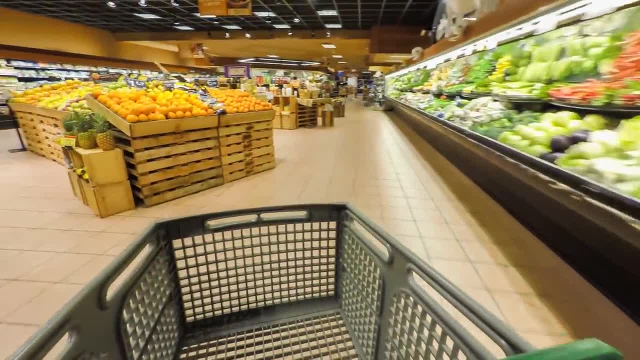 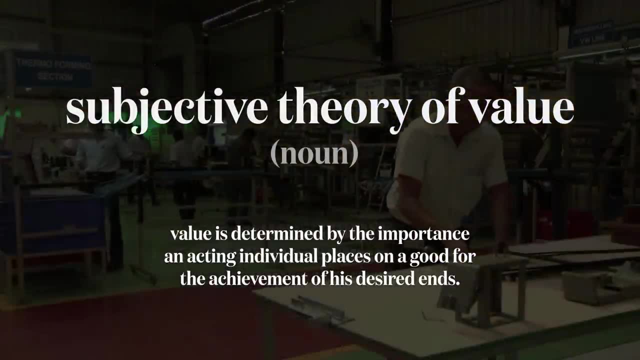 This deeper understanding in a world that was becoming more and more plentiful eventually culminated in the subjective theory of value. This theory argues that an item is not worth the sum of the materials and labour that go into making it, but rather it is a function of how important it is. 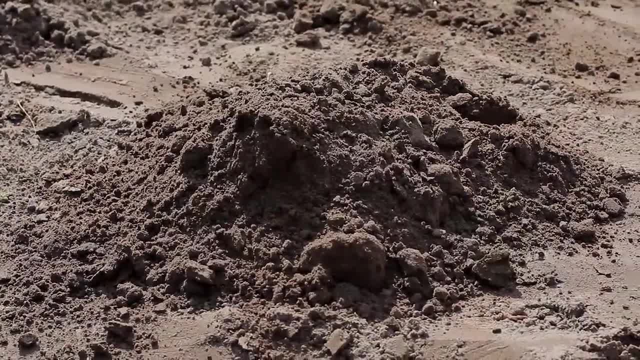 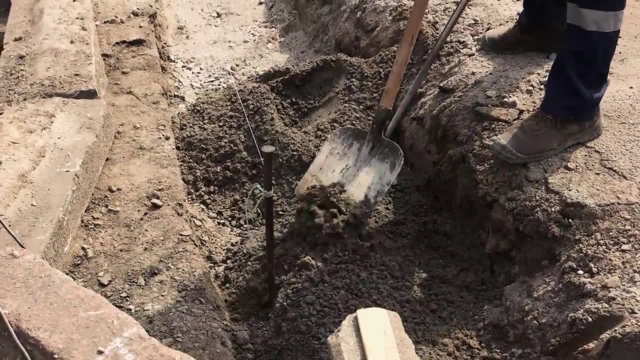 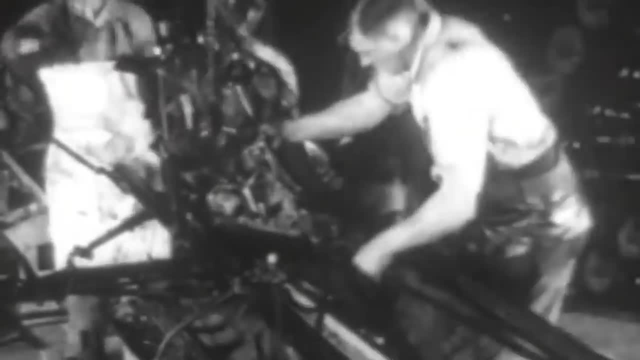 For example, a worker could spend their entire life digging the deepest hole in the ground the world has ever seen, but that hole is going to have less actual value than one that is dug 3 feet deep and hit a solid gold nugget. Or, as it relates to industry, a factory could build a car out of titanium, and sure it would. 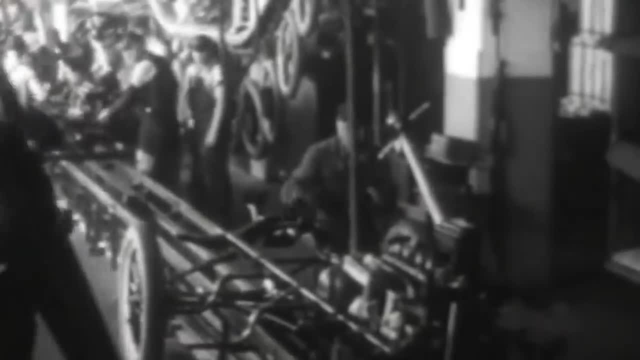 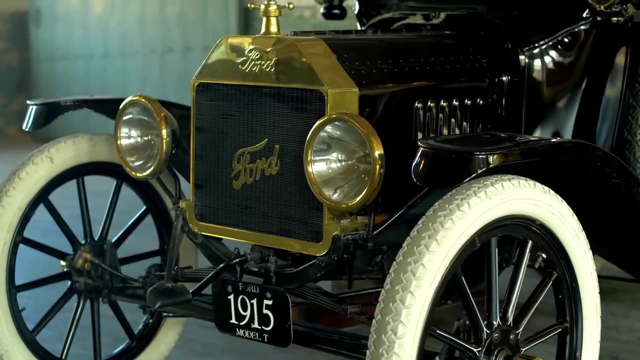 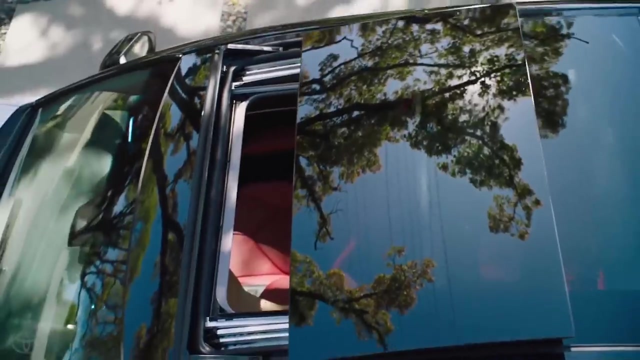 probably be a better car than one made out of steel, but it would take 10 times the man hours and 10 times the cost of materials to make that same car, and it might only be 20% lighter and stronger. Now, since people are not going to pay $300,000 for a titanium edition toyota camry, 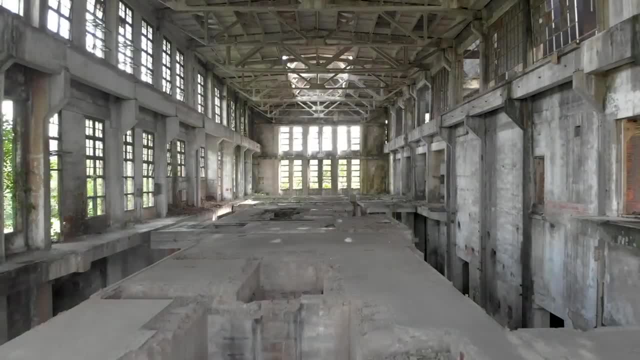 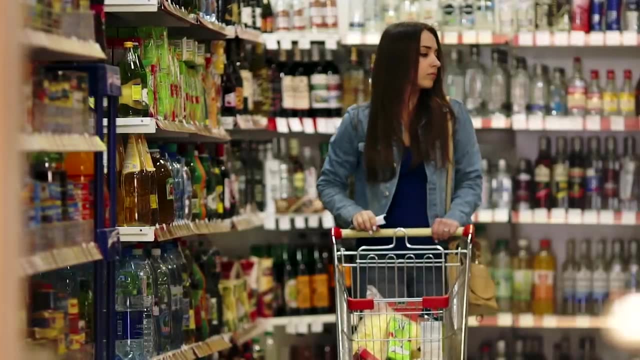 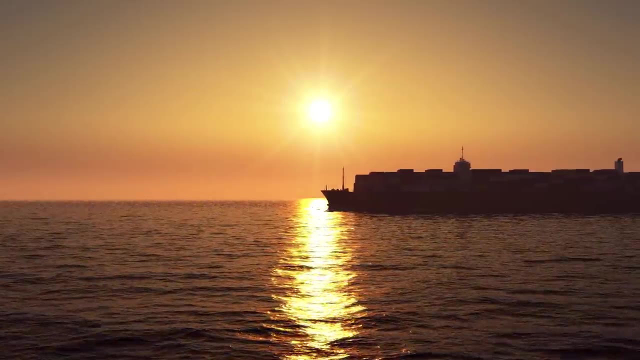 these types of subjectively inferior goods don't get made. Who is it that decides that these goods don't get made? Rational consumers. So suddenly the Austrian school of economics added a second role for the free market. Not only was it a medium of exchange that let people specialise and produce more, it also decided: 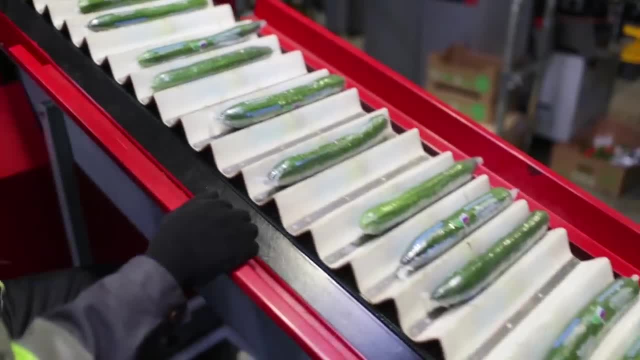 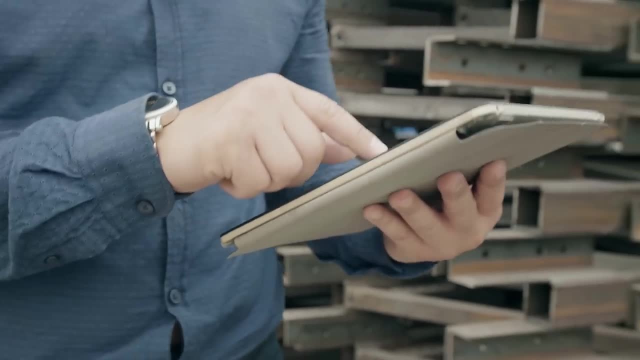 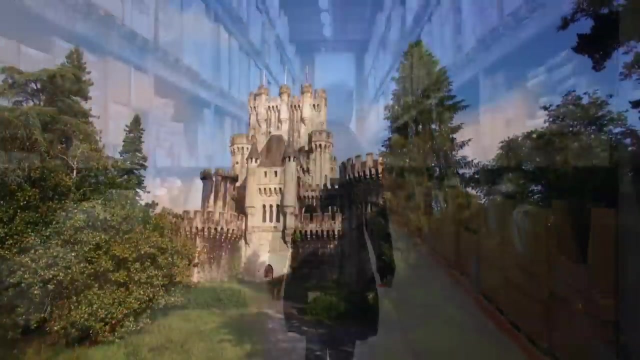 what it is that would be produced and what it is that would not. Suddenly, the most important thing in the world was not how much you could manufacture, but how carefully you could decide what to manufacture. Consumers were no longer units of labour. no, no, consumers were now king. 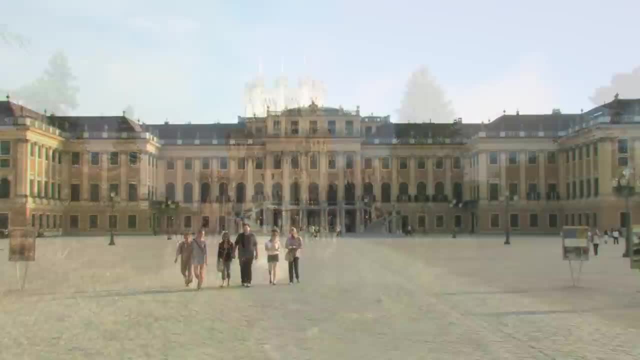 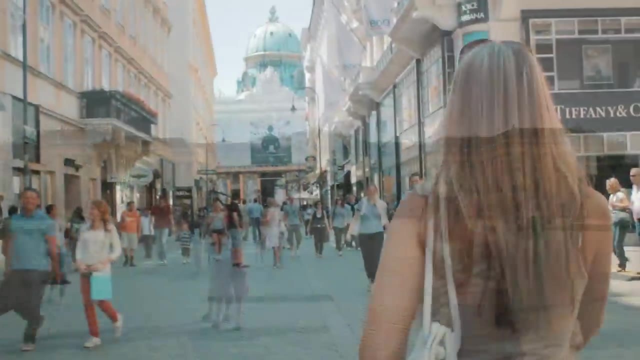 Austrian economics is today seen by most conventional economists as a very fringe ideology, for a few reasons. The first real reason is because, as we will see soon, consumers can be really dumb and irrational. It's no good to just give them free reign and hope for the best. 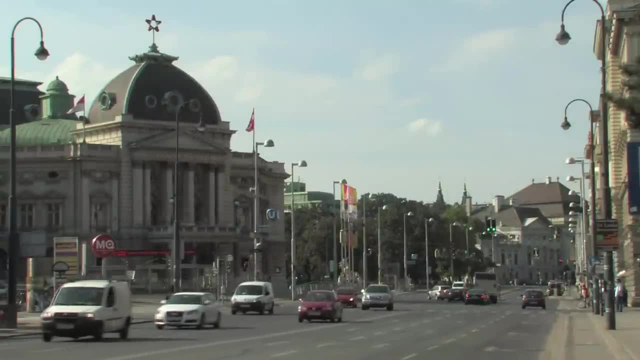 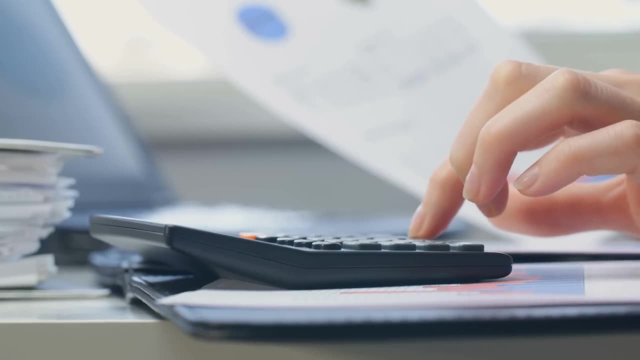 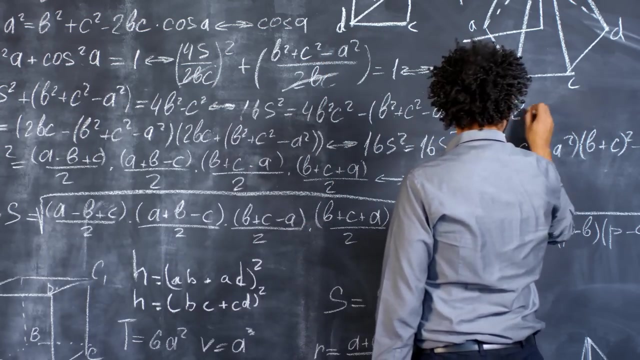 And secondly, it is very controversial because it relies very heavily on conjecture rather than rigorous mathematics or statistics. This makes a lot of their theories non-falsifiable, which in plain english means impossible to prove wrong, Which sounds great, but in reality it just means that, because there are no 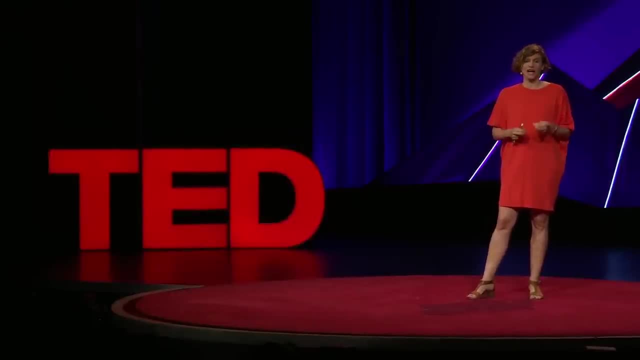 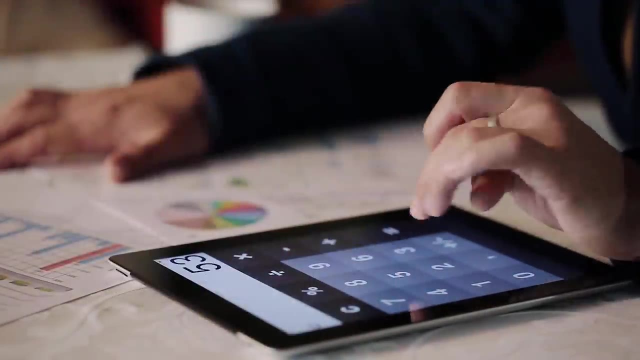 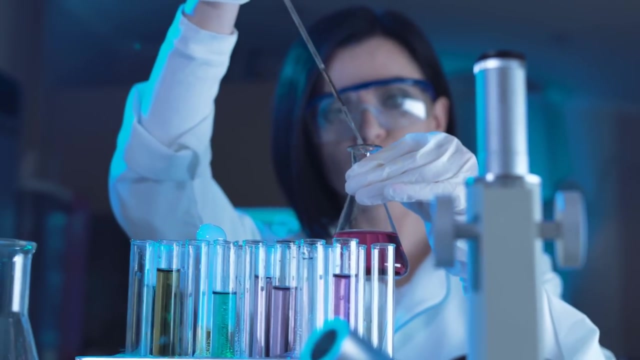 rigorous models drawn or prescriptions set, it's very hard to say that this outcome here proves something contrary to your theory. Now, because economics is a science, it is extremely important that all theories have a robust framework for being tested. You write a hypothesis, you conduct an experiment, measure the results and then record them. 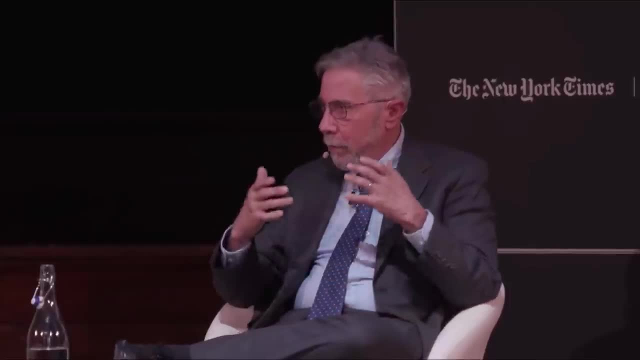 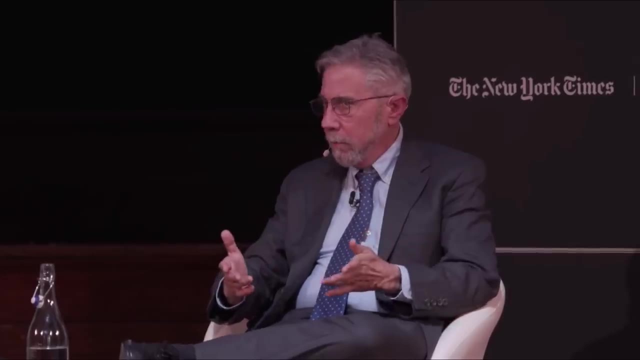 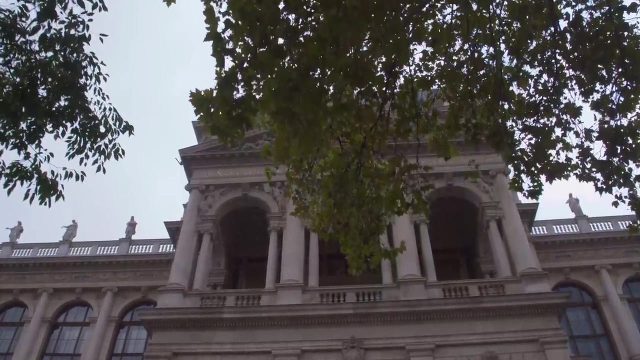 If you can't do that, then it's not science. For this reason, people like Paul Krugman have noted that Austrian economics is more a branch of philosophy rather than economics. Ouch, Outside of academics, the Austrian school remains really popular, in part because of its simple logical nature. 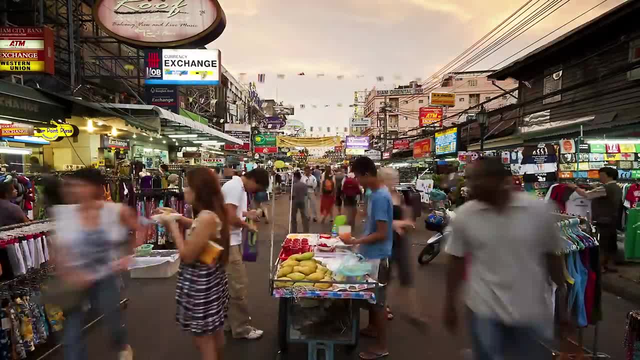 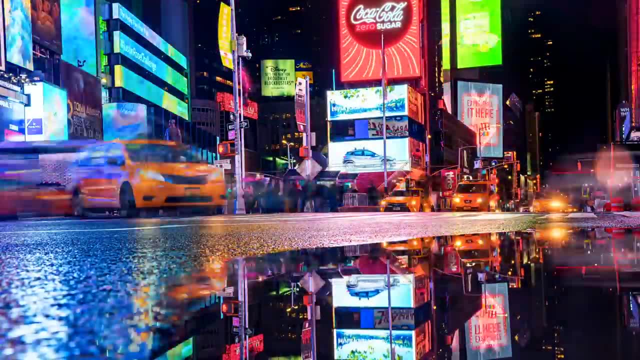 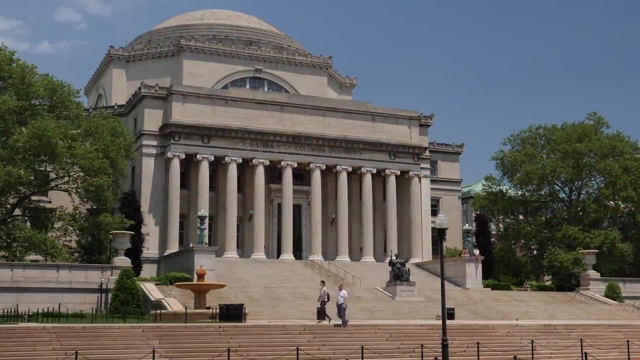 and in part because it tends to support free market principles, in part because it just does away with a lot of the modelling and mathematics that can make economics boring, and in part because it contributed a lot to our modern understanding of how the world works. Just because modern academic economists snob this school and its 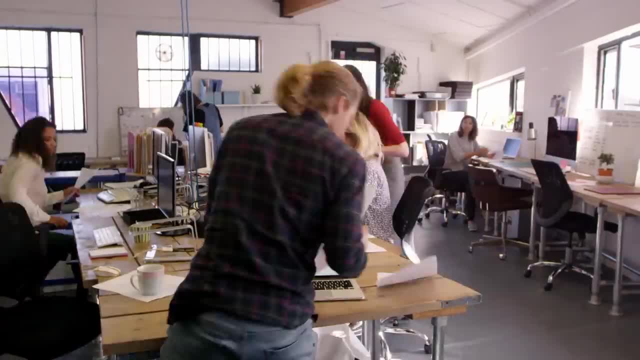 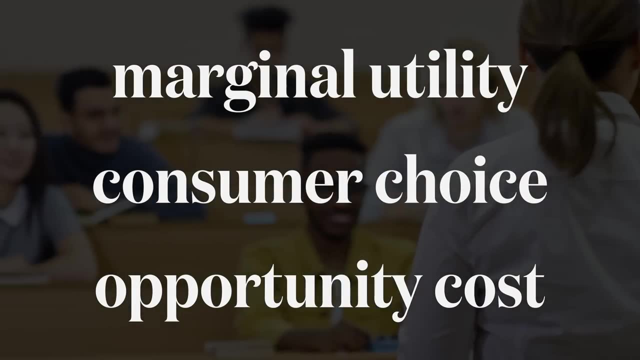 pundits does not mean that its contributions were any less important. Today. things like marginal utility, consumer choice, consumption and opportunity cost are the first things that students will learn in their introductory economics classes, But there are still ways to improve upon this and turn these understandings. 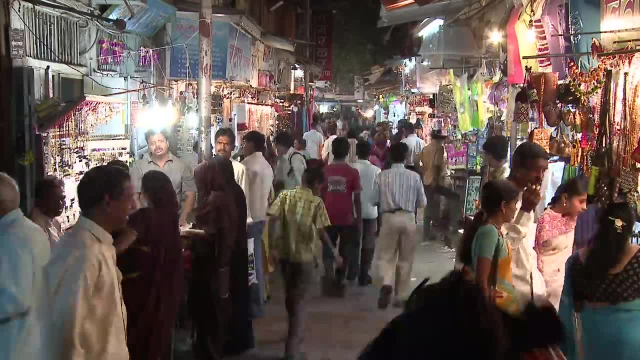 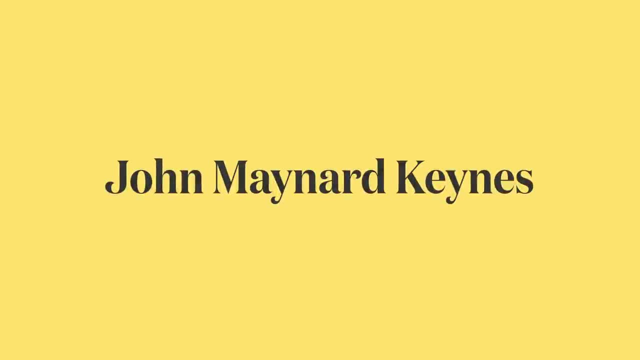 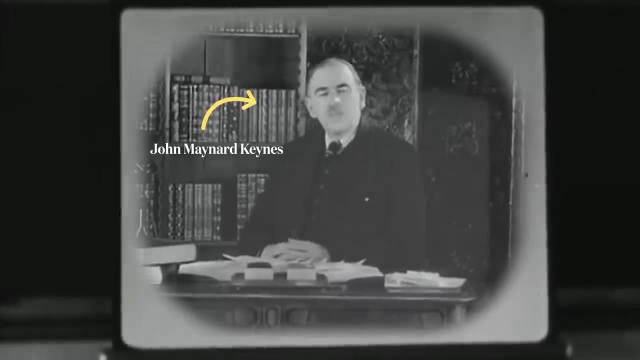 and insights into a workable framework for how to run a nation Outside of let people do what they do, Which is where John Maynard Keynes came in. If a regular person has heard of any economist, it would be Keynes. He is touted as the most influential economist of the 20th century and has today. 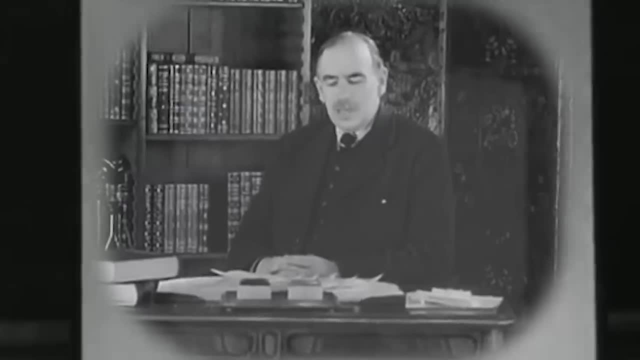 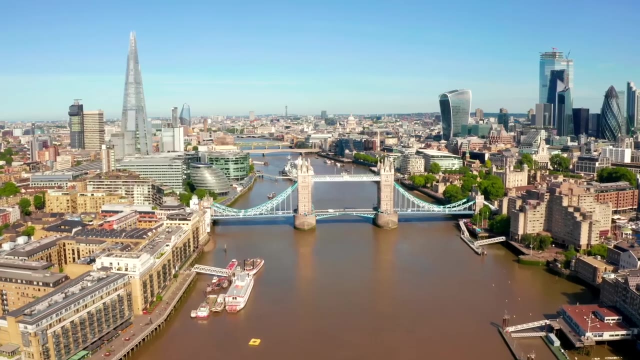 defined the way that almost all governments around the world manage their economic affairs. His contributions were plentiful and too extensive to explore in a single video, but one theory that was of particular importance during his lifetime was the introduction of counter-cyclical fiscal policy. 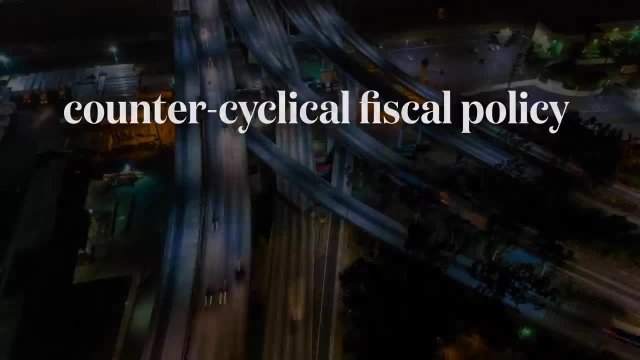 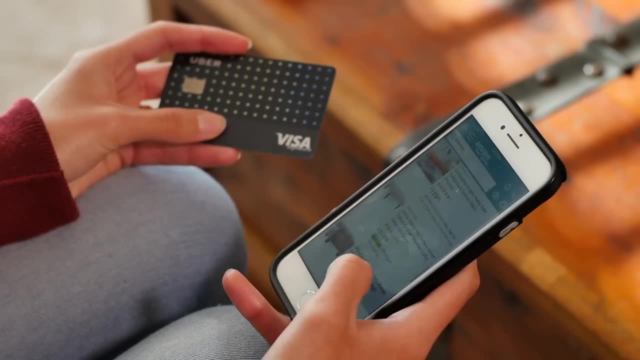 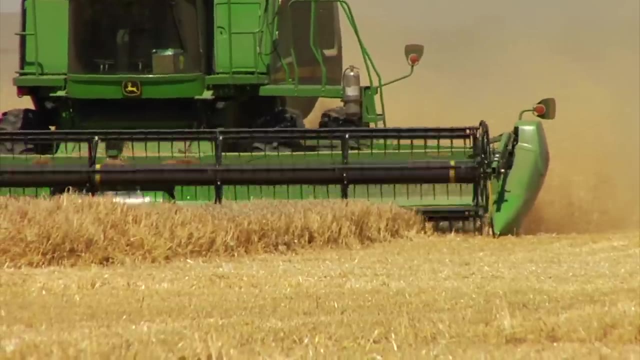 Since the rollout of classical economics and the wealth of nations, economies have become many, many times more complex. Factories, markets, advanced financial systems, consumer debt, public corporations were all now common place. The ebbs and flows of national prosperity were no longer determined by the harvest. 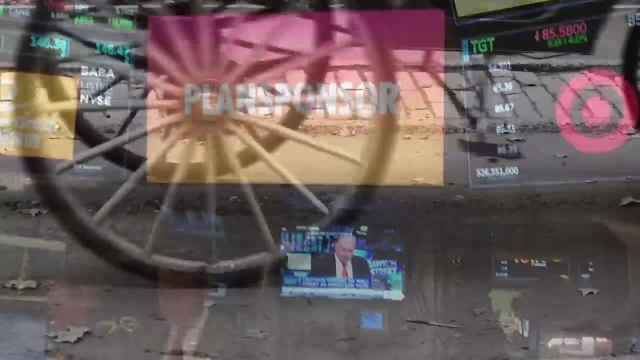 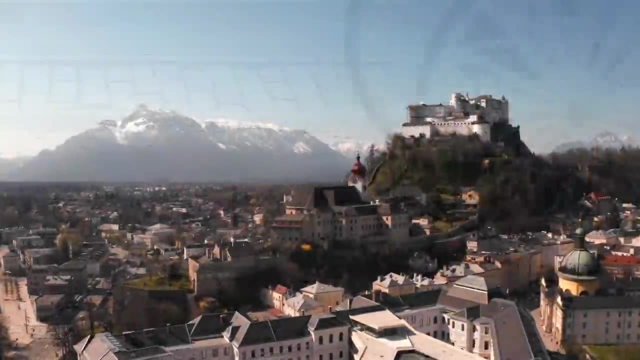 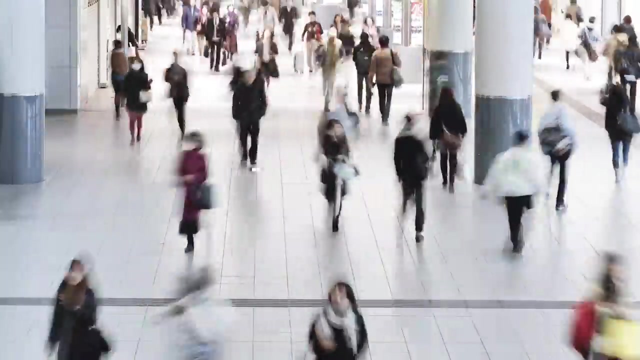 but rather by the business cycle. Around the early 1800s, economies started experiencing ups and downs that could no longer be explained exclusively by outside forces, but rather by the sentiment of the people within the nation. Since consumers were now the centre of modern economies, their feelings 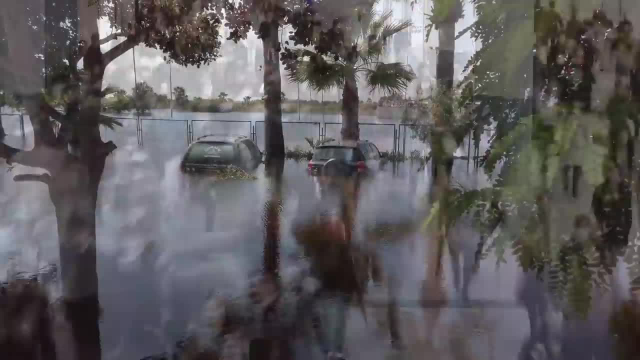 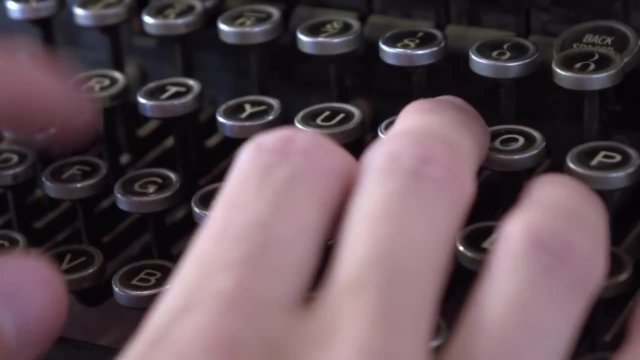 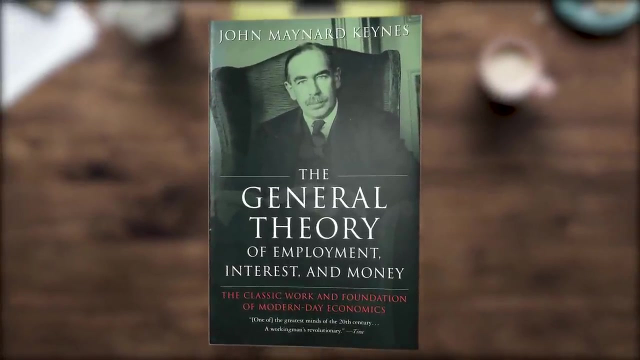 impacted the economy as much, if not more so, than real forces like natural disasters, wars or plagues. This again shows that this school of economic thought was the product of its time. Keynes started writing his most widely recognised work, the general theory of employment, interest and money, during the great depression. 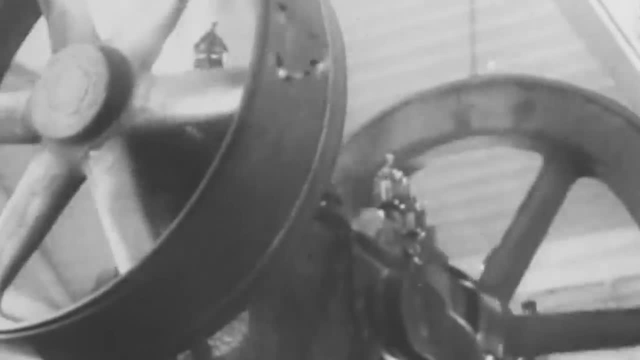 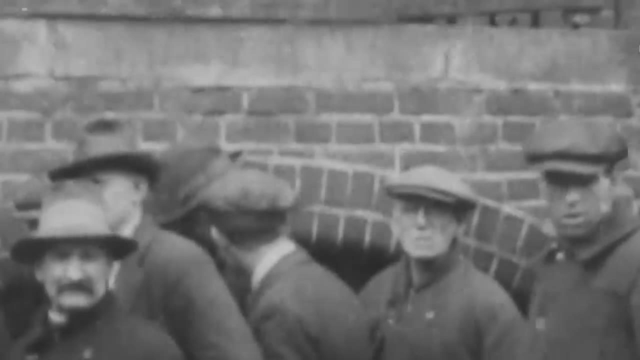 These types of ups and downs could be very unsettling and could impact the health of an economy in the long term. For example, who would want to invest in a company if they knew a devastating recession was going to come about every 10 years, which would probably send 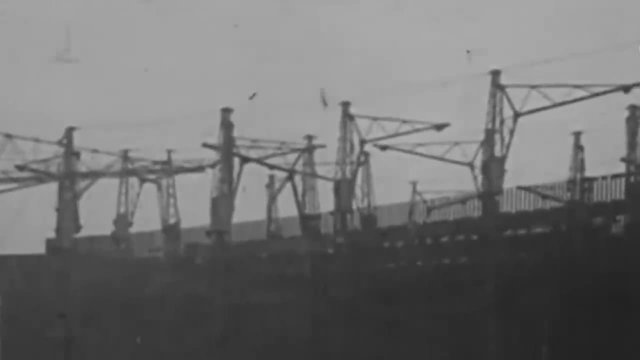 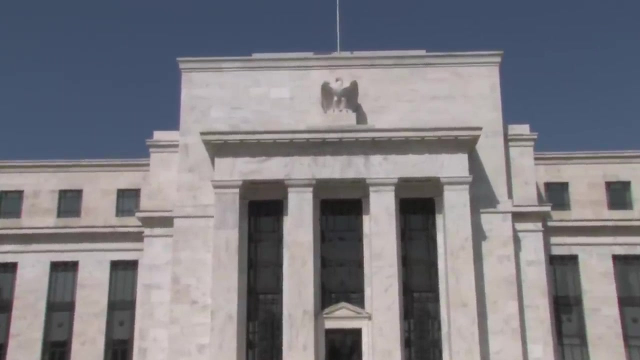 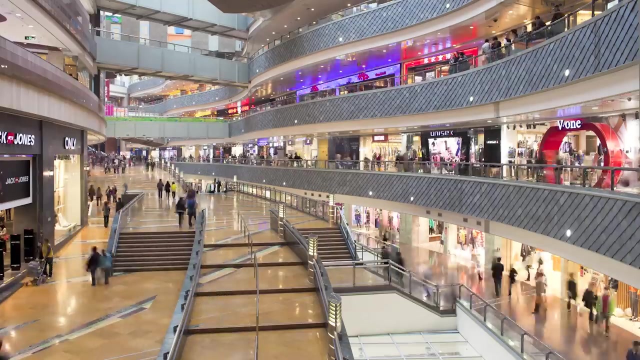 that business bankrupt? well, nobody, But businesses need funding to continue to grow and contribute to the economy. The solution was to try and smooth out the business cycle by artificially influencing the spending of consumers. Nations would do this through fiscal policy, which called for taxing people more and spending less. 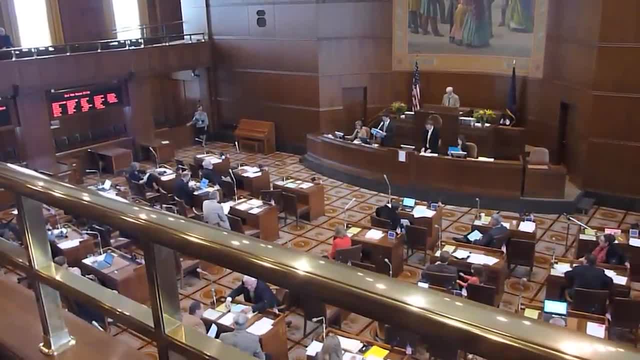 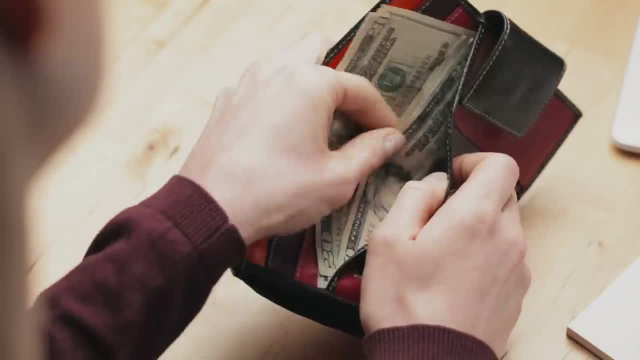 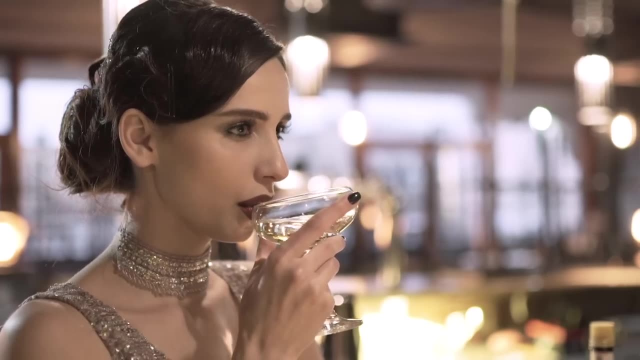 people into having less money, which means they can't go quite as crazy with their spending and taking on of debt, making the good times not quite as crazy, conspicuous and Gatsby-esque. On the flip side, when that tax is lowered and the government starts spending lots and 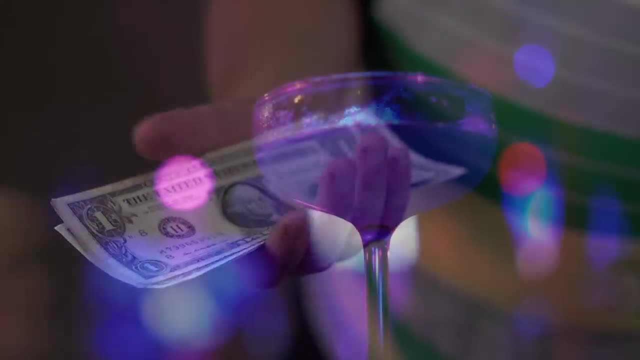 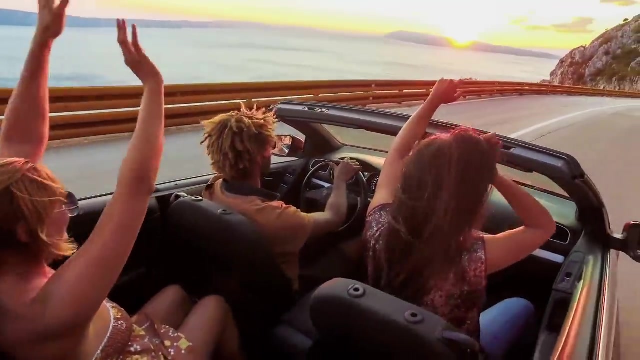 lots of money. well, suddenly you have a whole lot of extra money in your pocket that you can go out and spend to make the economy not as terrible. during a recession, Keynes' plan was not to completely remove the business cycle, but to make it go from. 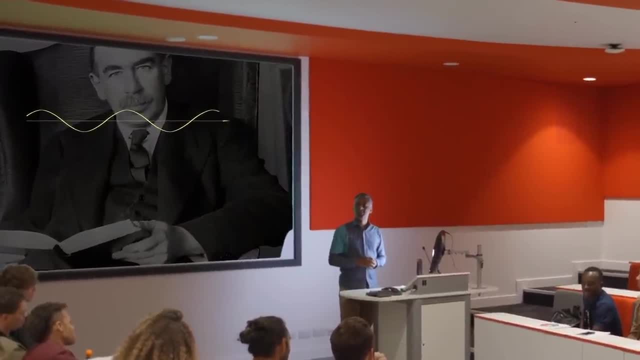 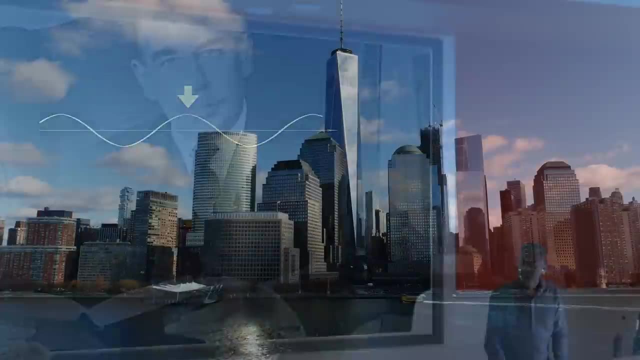 looking like this to like this. The benefits of doing this are kind of hard to see. Sure, the bad times are not as bad, but the good times are not as good. So what gives? Well, the argument is that by making both of these less severe, the economy was more. 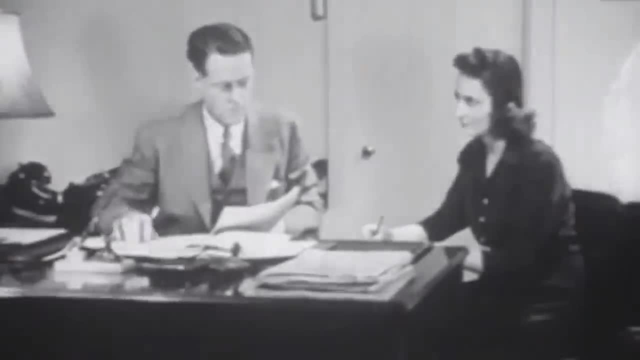 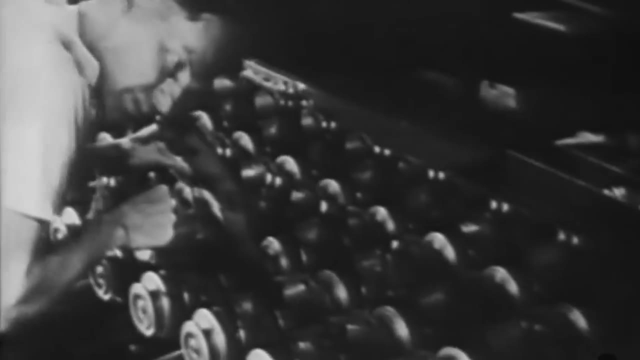 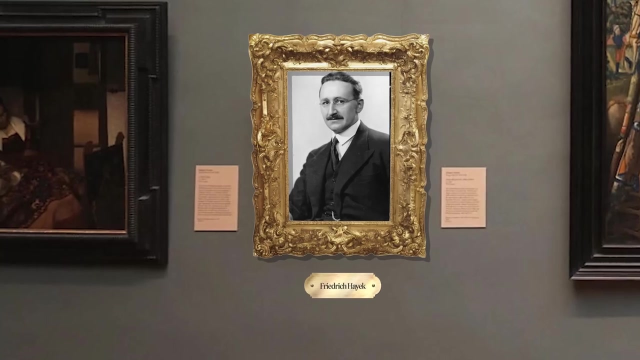 consistent and people could plan for long term growth rather than just surviving the next catastrophic downturn. The Austrian school hated this idea. It was tampering with the free market, which would limit efficiency. These disagreements often saw Keynes at odds with his Austrian contemporary, Friedrich Hayek. 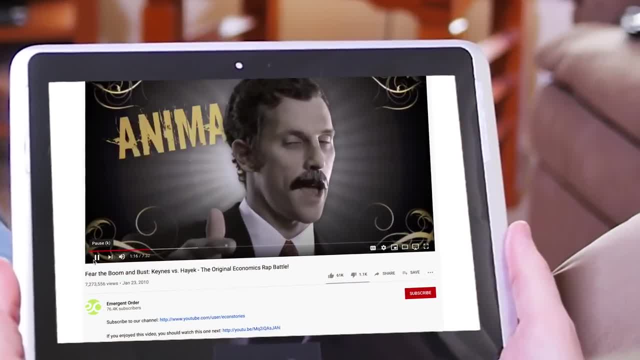 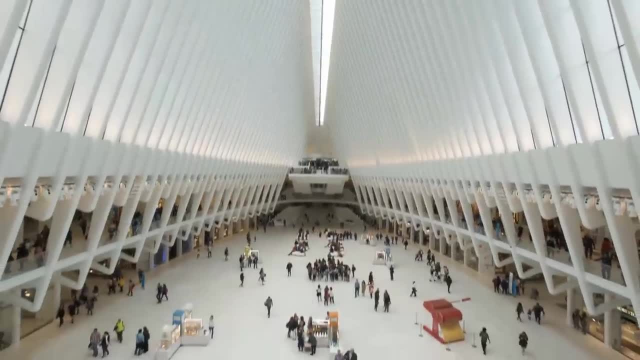 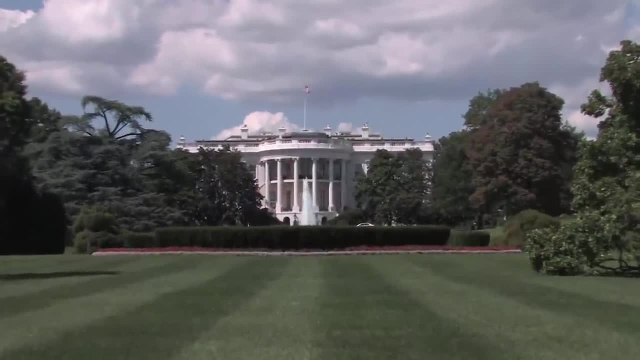 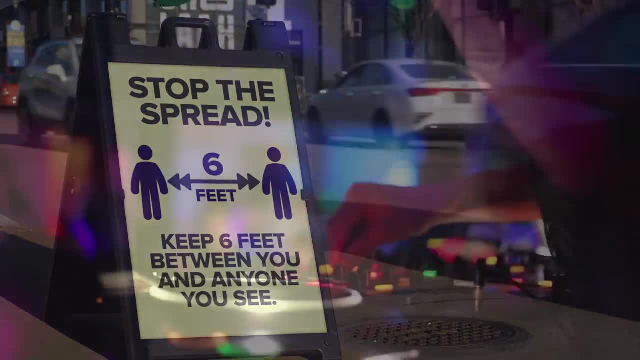 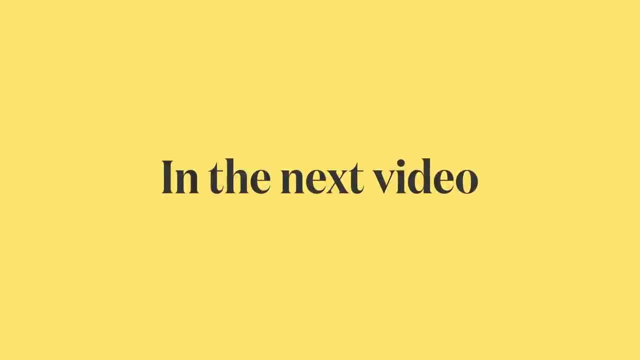 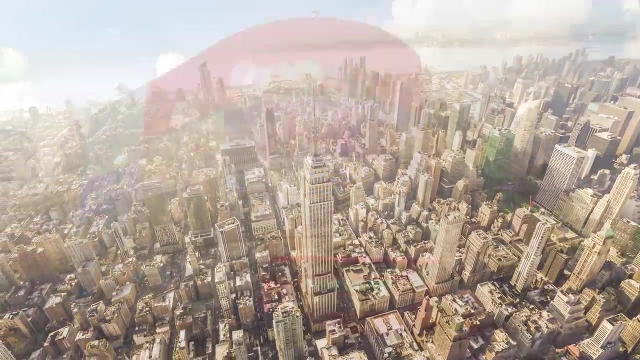 very quick to roll out Keynesian fiscal stimulus during a downturn, but normally forget about higher taxation and lowered spending during the good times. Economics is a very diverse study that is founded on an unanswerable question. By its very nature, it is going to cause some disagreements, conflicting ideas and other. 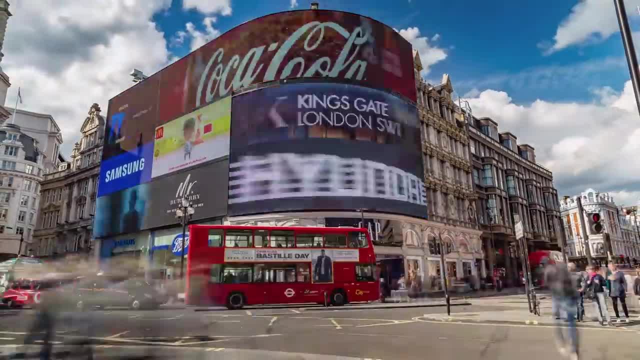 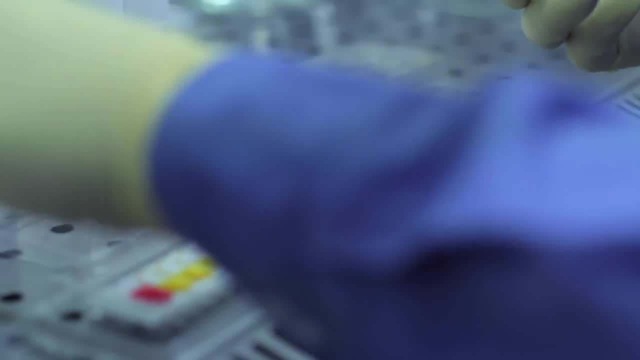 ideologies, yes, even some controversy. Now, this is not that much different from any other scientific pursuit. If you ask any group of scientists about a new theory in their respective fields, they are all going to have very different opinions on it. It's just that. 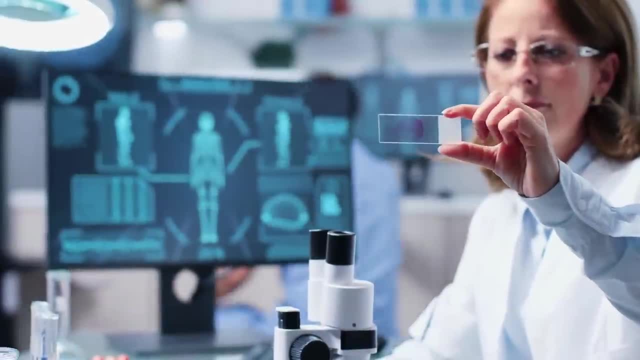 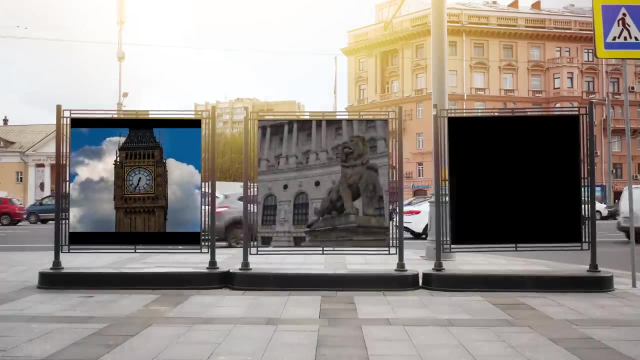 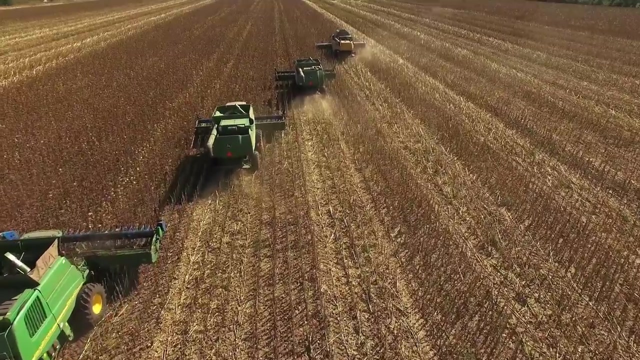 the opinions of economists garner a lot more attention because in many ways it is us who is being experimented on. These three schools of economic thought- classical, Austrian and Keynesian- agree on far more than they disagree on, but, as with any competing ideologies, they are defined. 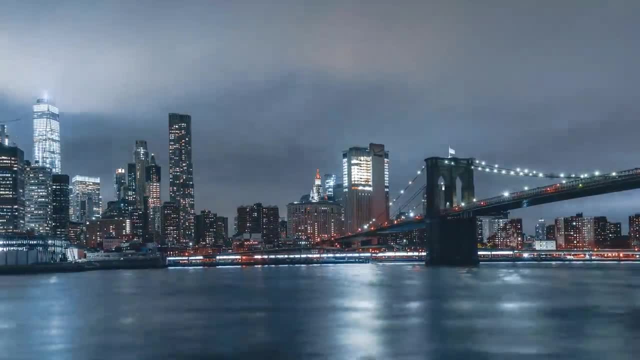 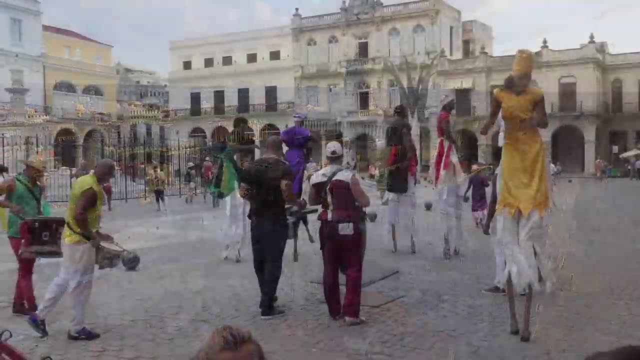 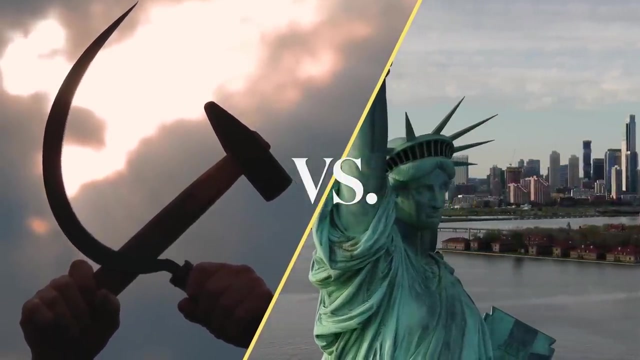 by their differences. Now, so far as we have seen, these have been more of an evolution on one another rather than a revolution. Now revolution segues us nicely into the next video in this series: Marxism vs Lazy Fair Capitalism. But for now, at least remember that amongst all of these, 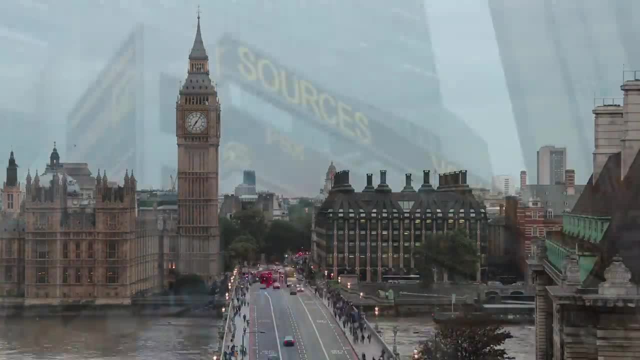 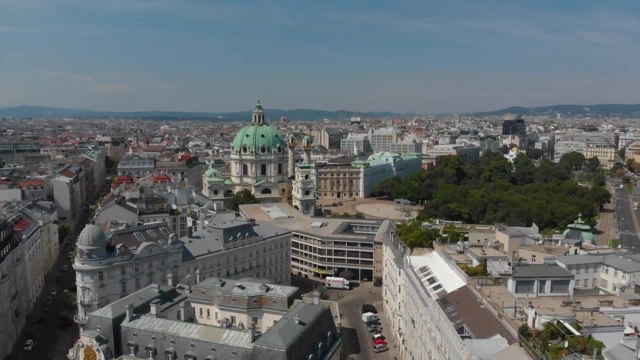 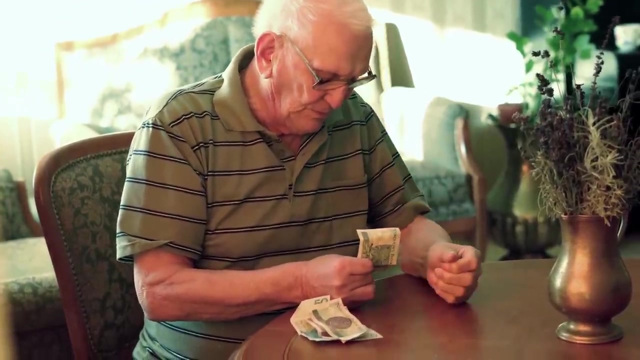 disagreements, economists are still working towards a common goal: solving the central economic problem. They agree on far more than they disagree on, and one thing that everybody can agree on is the importance of investing in your future. That's because there are few things in life that are scarier than reaching retirement and having 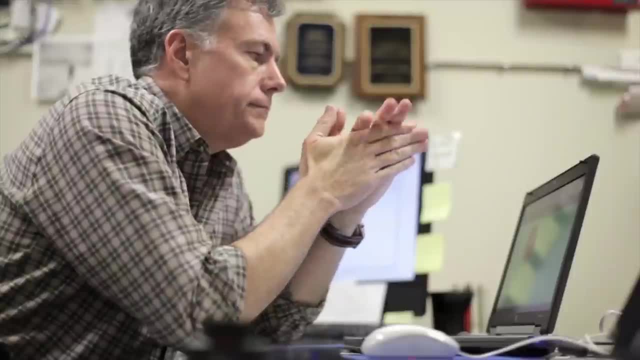 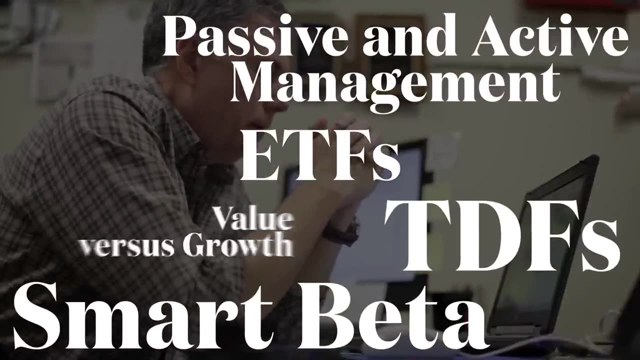 to worry about having enough. Making matters worse. getting started with investing can be intimidating due to arcane words like ETFs, TDFs, smart beta, passive and active management, value vs growth, volatility and momentum strategies, to list just a few. 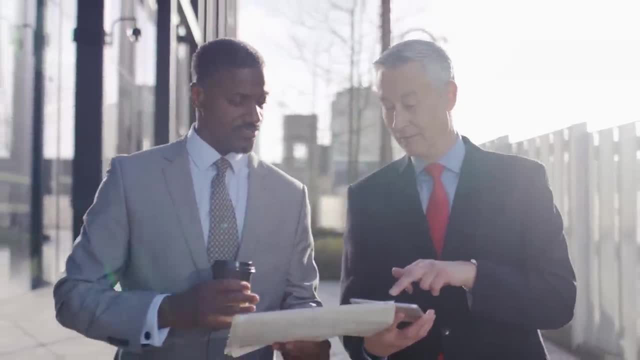 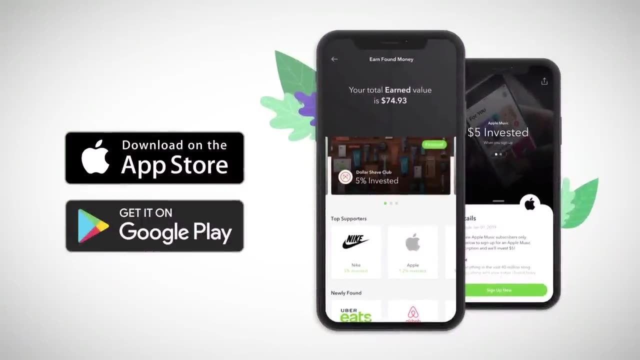 Fortunately, you have a friend in the investment business, one that we trust our money here with at Economics Explained, and that friend is Acorns. Acorns is your all-in-one financial services app that makes investing as easy as spending Every time you use your debit or credit card.